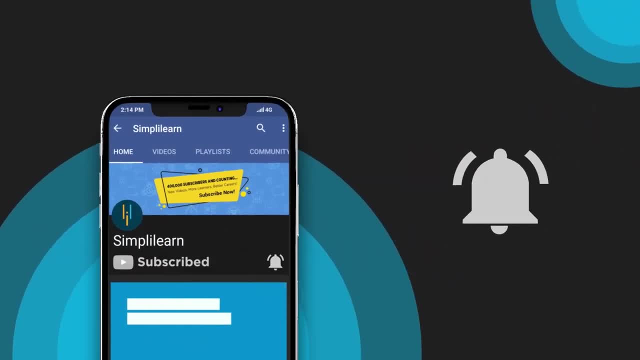 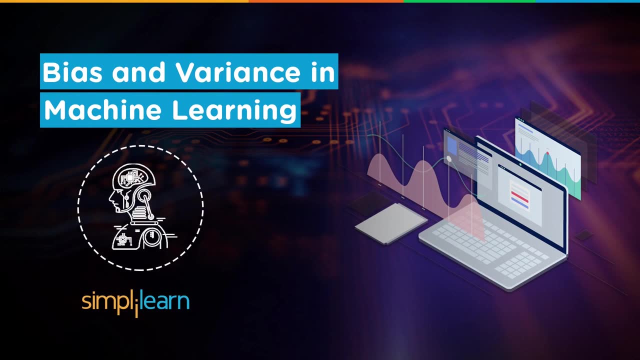 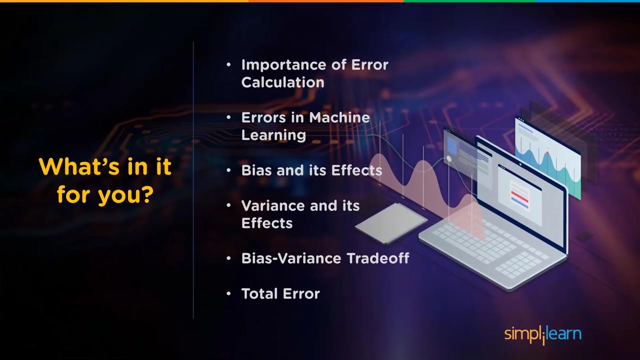 Bias and Variance in Machine Learning. Welcome to Simply Learn. My name is Richard Kirshner, with the Simply Learn team. That's wwwsimplylearncom. Get certified, Get ahead. What is in it for you? Importance of Error Calculation. Errors in Machine Learning. Bias and its Effects. Variance and its Effects. Bias Variance, Tradeoff, Total Error. 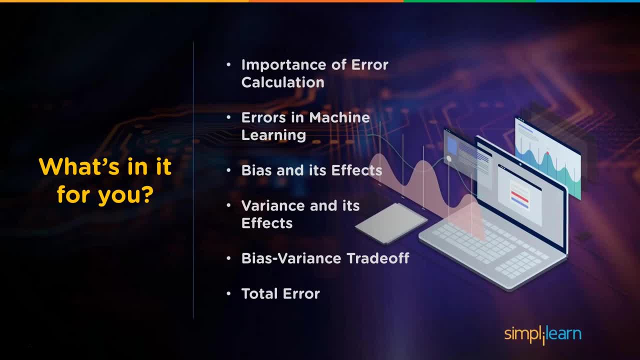 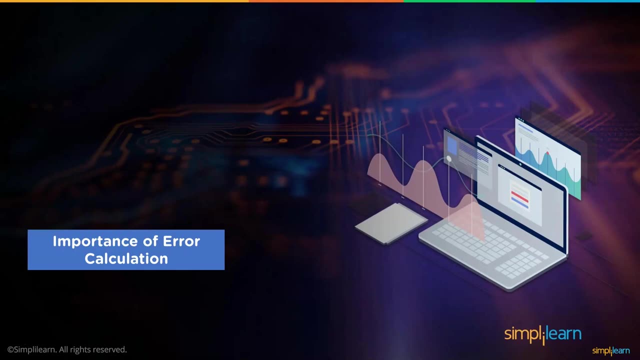 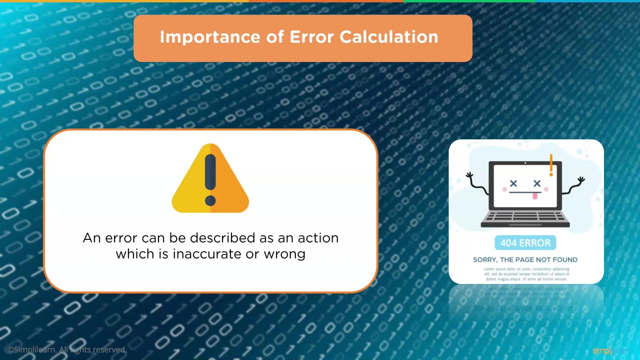 Really we're starting to dig in deep into our different machine learning models so we can understand which ones work better and why. And very central to that is the bias and the variance and how, these effects and the tradeoffs. Importance of Error Calculation. Importance of Error Calculation: An error can be described as an action which is inaccurate or wrong. 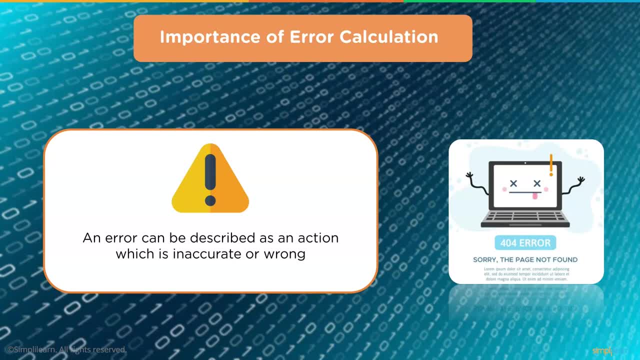 You see here everybody's favorite or least favorite error: 404 error trying to find a website. Sorry, the page cannot be found. So this is really what we're looking at is, where do we find things that are wrong, because we don't really want our errors to rule our models. 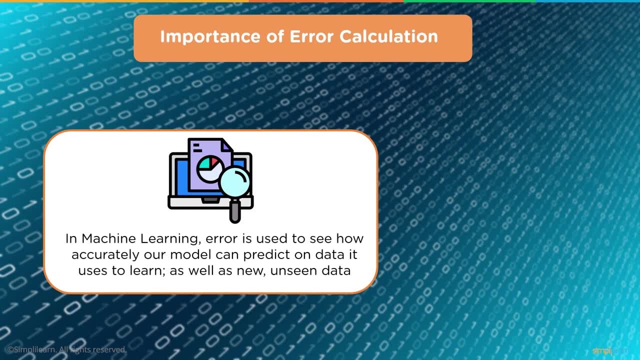 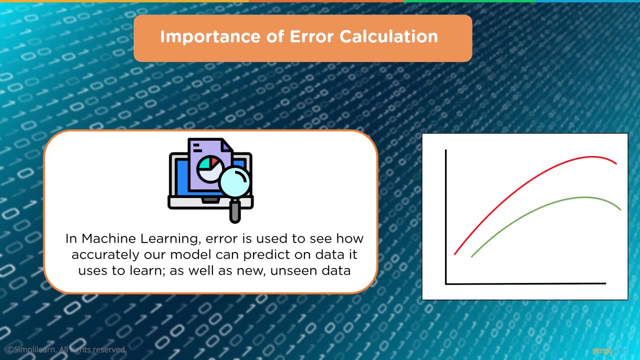 And in machine learning, Error is used to see how accurately our model can predict on data it uses to learn, as well as new unseen data. And you can see here we have a nice little chart: model, predictions, actual values and the error. So the error being the difference between the two. 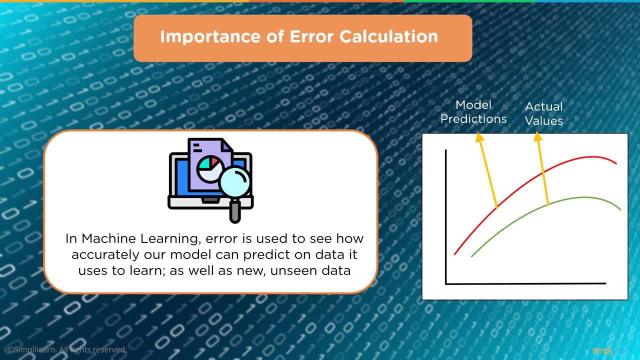 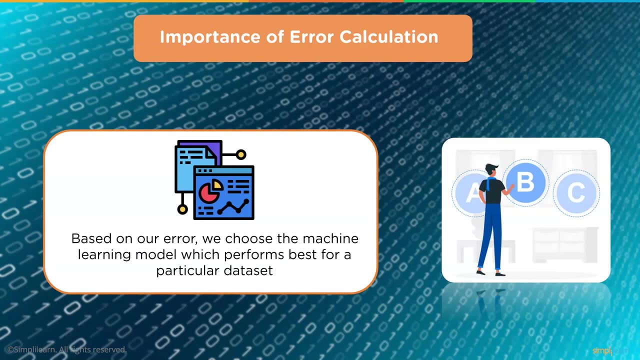 This little chart. it's usually a plus or minus kind of thing. We talk about errors if we're doing regression models, or it could be in this case, how many mispredicted values if you're doing categorizing Based on our error. we choose the machine learning model which performs best for a particular data set. 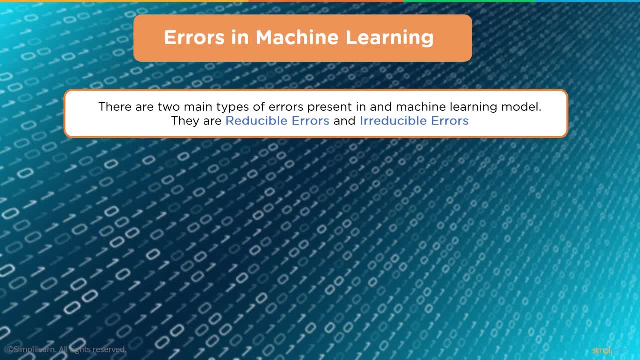 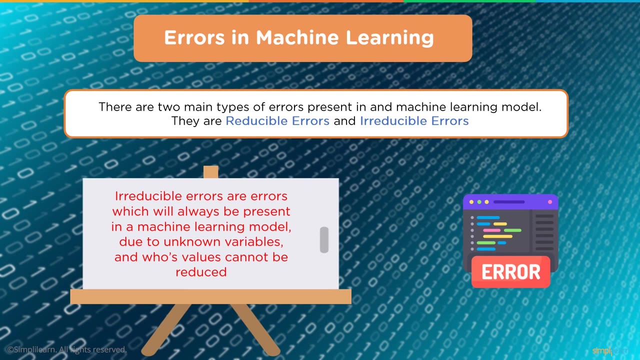 And so let's go ahead and dig a little deeper into errors in machine learning. There are two main types of errors present in a machine learning model. They are reducible errors and irreducible errors. Irreducible errors are errors which will always be present in a machine learning model due to unknown variables and whose values cannot be reduced. 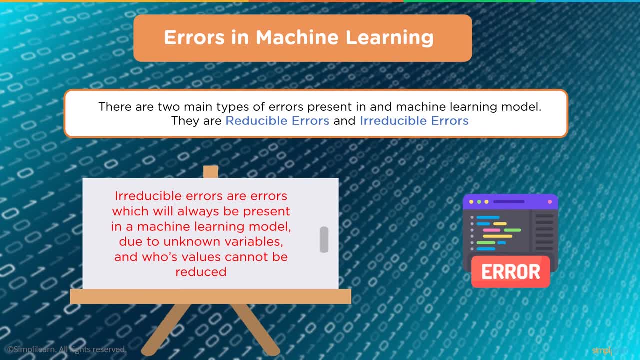 You can think of this if you're trying to guess wind direction and how heavy the wind's going to blow. It's really hard to do. It's really hard to see something. There's something even as humans, we can't predict because of the chaos. and so you have that part of the error, that irreducible error, that you're never going to be able to be 100% perfect on your predictions. 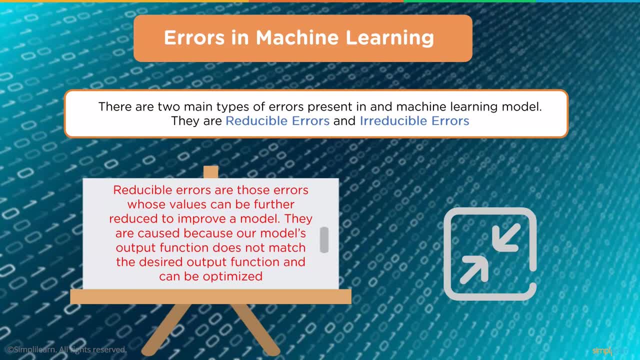 Reducible errors are those errors whose values can be further reduced to improve a model. They are caused because our model output function does not match the desired output function and can be optimized, And so you can think of reducible error as something we can try to address and fix. Irreducible means that there's 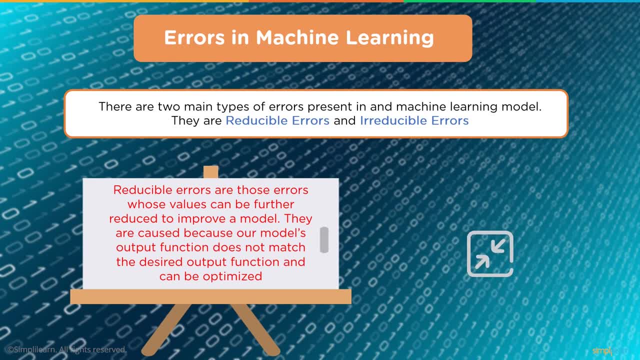 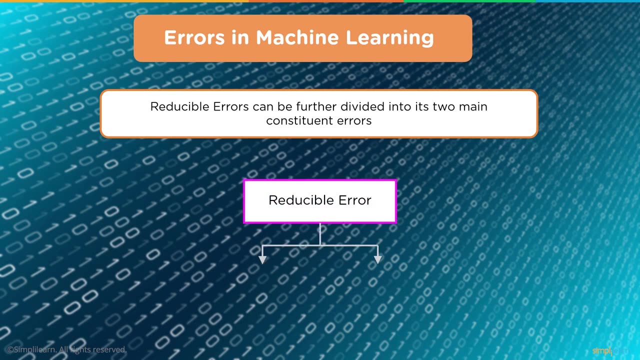 just, it's just beyond the capacity of the computer to do, It's beyond the capacity of anybody to do, because there's always some form of chaos involved in any system. So you're never going to be 100%. no errors. Reducible errors can be further divided into two main constituent errors. We have bias. 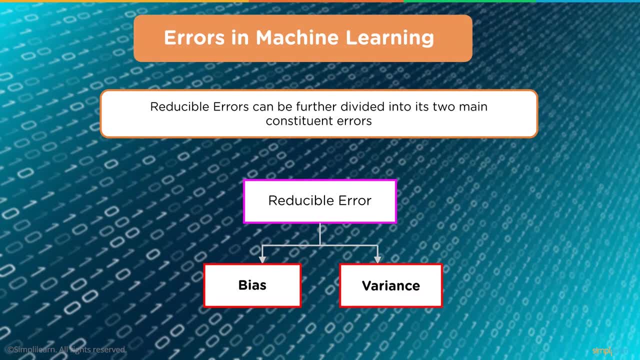 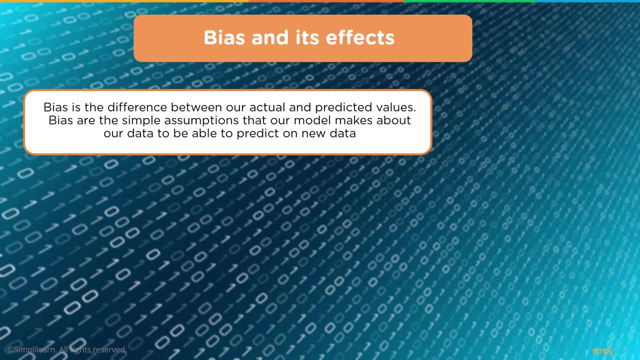 and we have variance. So now we're talking about very specific types of errors. We're looking at the bias and the variance, And let's start with bias and its effects. Bias is the difference between our actual and predicted values. Bias are the simple assumptions that our model makes. 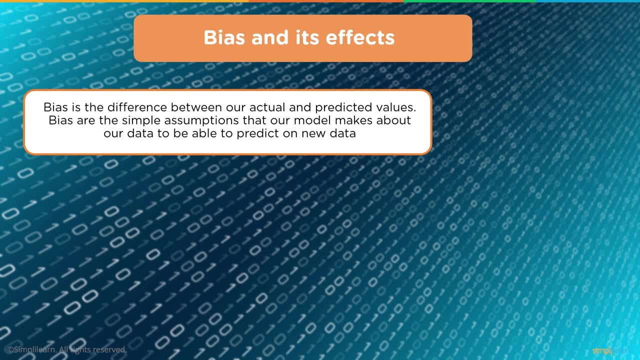 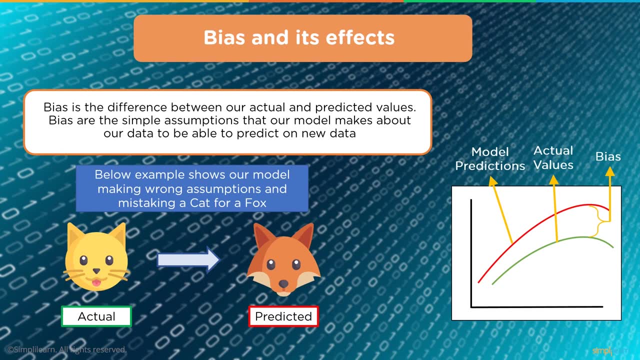 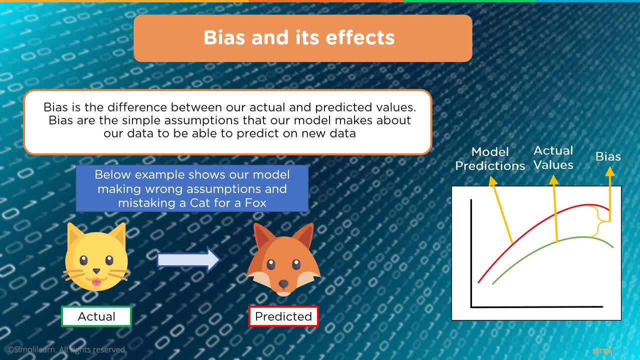 a false and we have a false, So we have a false and we have a false, So we have a false. There are Honduran letters. You have to be lucky, because that is what the class voll someday T 하나� and plus scales, and that arrow is a. 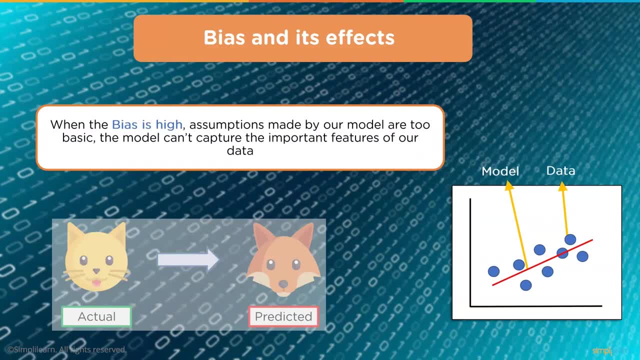 a s x made by our model are too basic. The model can't capture the important features of our data. One of the early facial recognition softwares that were out there based the recognition pattern on the person's profile only and not their facial features, And so we had a huge bias as far as certain people and 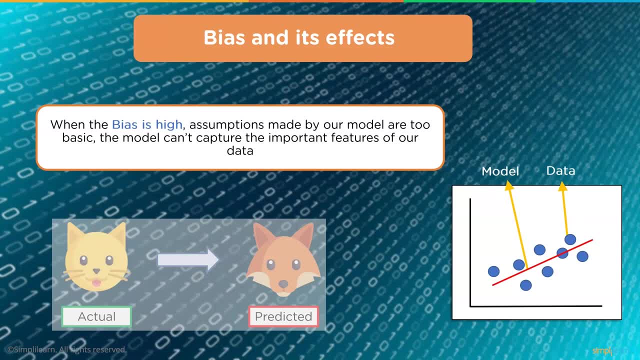 because their profile matched and it didn't go any deeper than that. That's a kind of thing. and you can see, of course, the cat and the fox. they both have pointed ears- probably not, you know. that's kind of generates a bias for pointed ears to foxes or something. And so we look at our model and our data. we 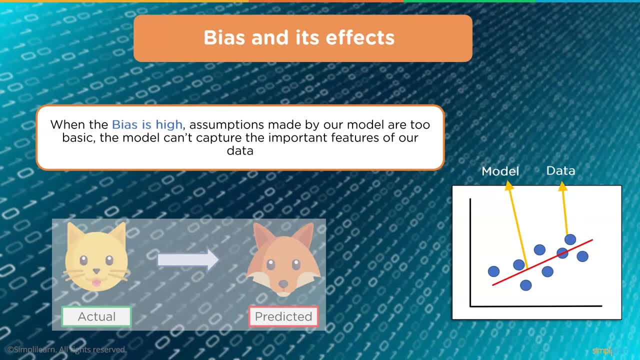 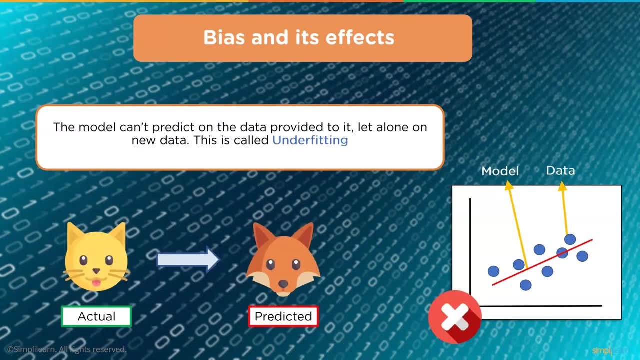 start realizing that we need to get a little deeper and look a little bit more finite details, or the model needs to program itself and look a little closer. what it's looking at, The model can't predict on the data provided to it, let alone on new data. This is called under fitting, So there's our key word for this. 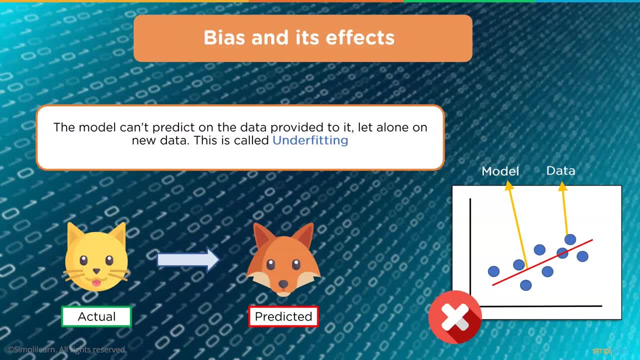 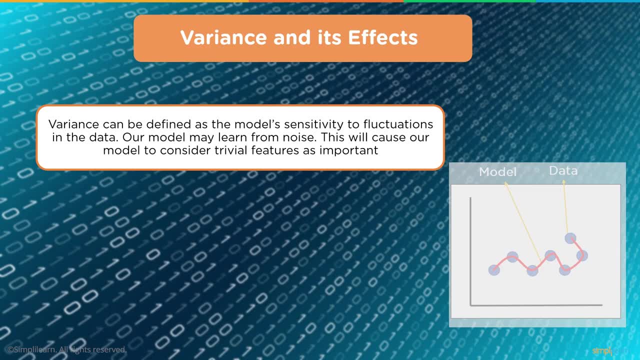 particular kind of bias is an under fitting effect, is it's not able to predict something because it doesn't look at all the different features, Variance and its effects. Variance can be defined as a model sensitivity to fluctuations in the data. Our model may learn from noise. This will cause our 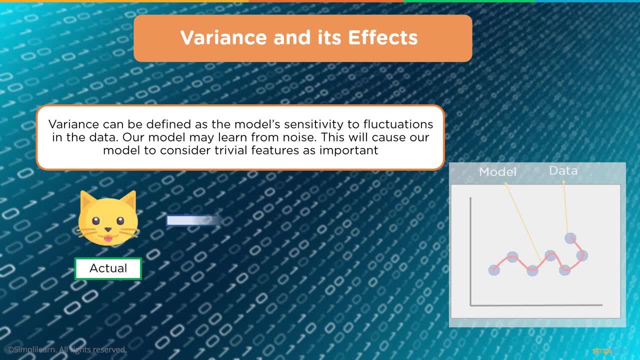 model to consider trivial features as important, And so we can start looking at. here's our actual and our predicted value. You can see where the cat becomes a cat, the fox becomes a cat and it might be looking at the fact that the nose and the ears, It might be looking at very specific features and saying, well, 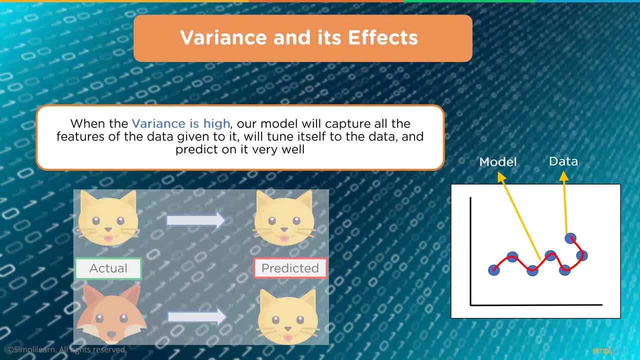 that defines whether it's a cat or a fox. When the variance is high, our model will capture all the features of the data given to it, Will tune itself to the data and predict on it very well, And this is a very important thing to note. 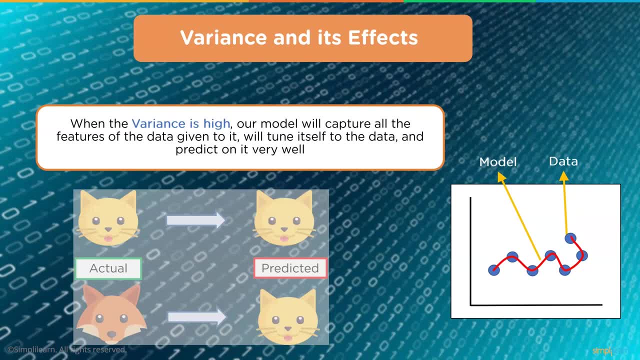 It's kind of hard to visualize. So the model will capture all the features of the data and it predicts very well. So our model comes out really good on the data that we programmed it with. It knows it. it's almost like a hundred percent. 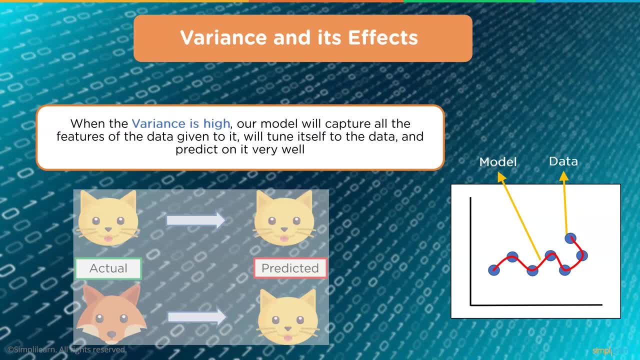 When you put new data in, it doesn't do as well- And that's when you know you've overfitted- is the data you did not train it with doesn't show up correctly. New data may not have the exact same features and the model won't be able to. 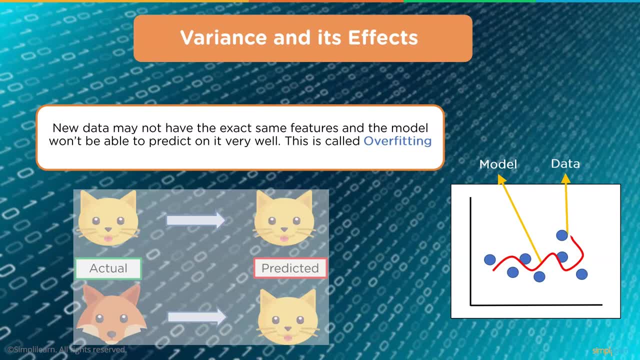 predict on it very well. This is called overfitting. So remember, underfitting kind of looks at just like a generic profile of it and it's not trained well enough. Overfitting is the opposite. It's so trained to the data there's looking. 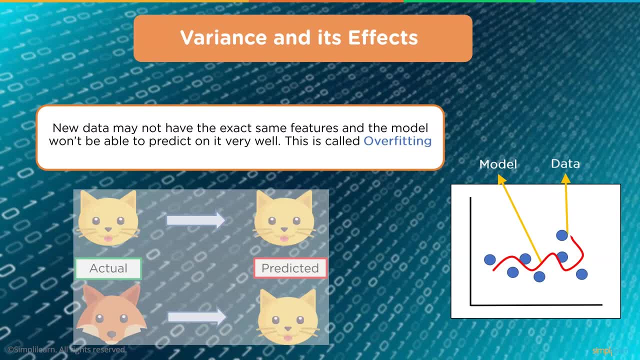 for very exact outputs Based on the data coming in, And in fact, there's now a number of models out there that when they do the fitting, they stop when they look at the data that's not being used as a training model And they'll just automatically stop when the 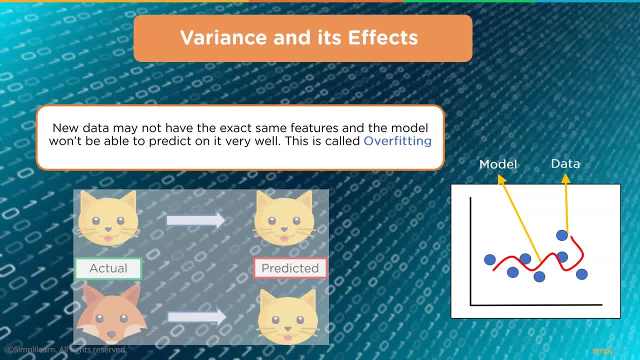 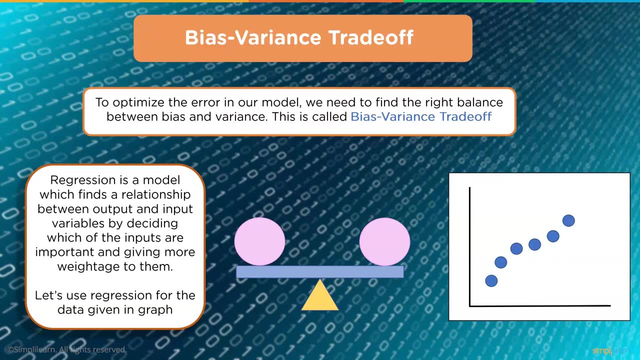 two kind of match When you have, the amount of error is about the same between them. So we have a bias variance trade-off And we talk about bias variance trade-off To optimize the error in our model. we need to find the right balance. 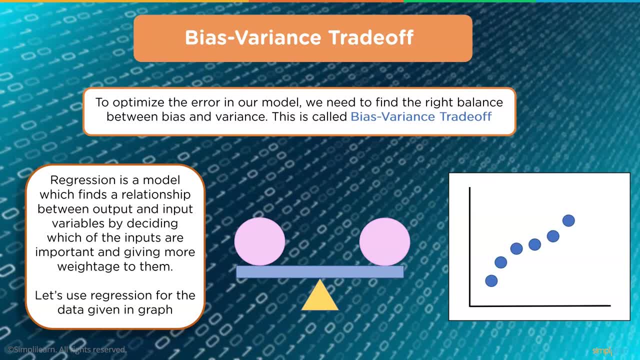 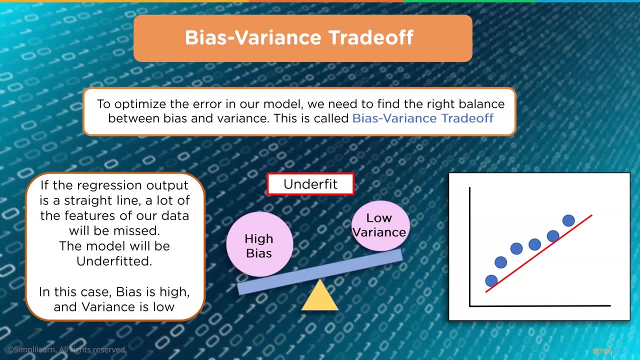 variance. This is called bias variance. trade-off Regression is a model which finds a relationship between output and input variables by deciding which of the inputs are important and giving more weightage to them. Let's use regression for the data given in the graph. The regression output is a straight line A. 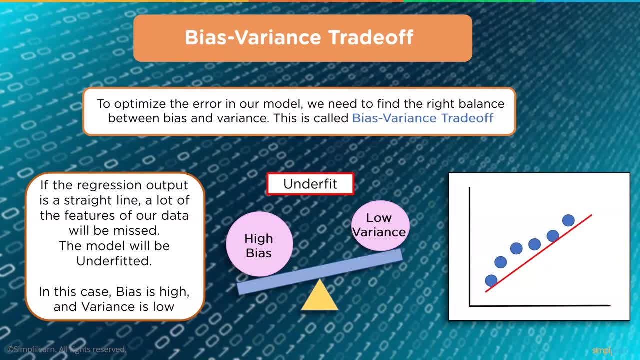 lot of the features of our data will be missed. The model will be underfitted. In this case, bias is high and variance is low, And you can think of it this way is that you have a high error on everything, So your your error on both. 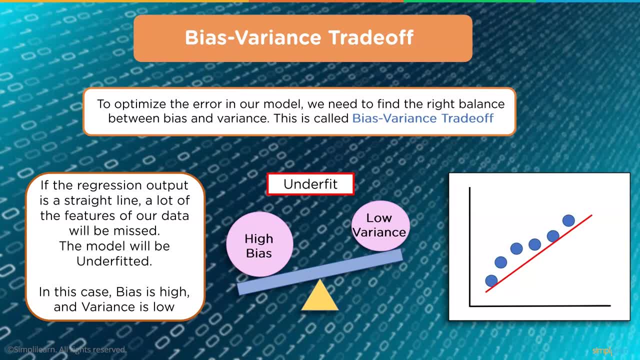 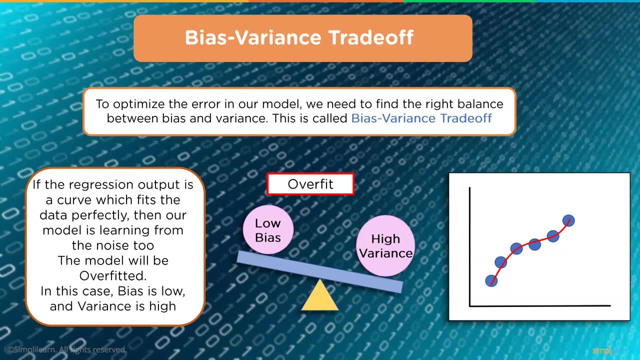 the data you're fitting it with and on your output is still high. If the regression output is a curve which fits the data perfectly, then our model is learning from the noise too. The model will be over fitted. In this case, bias is low and variance is high. If you think of our cat and fox example, the noise might. 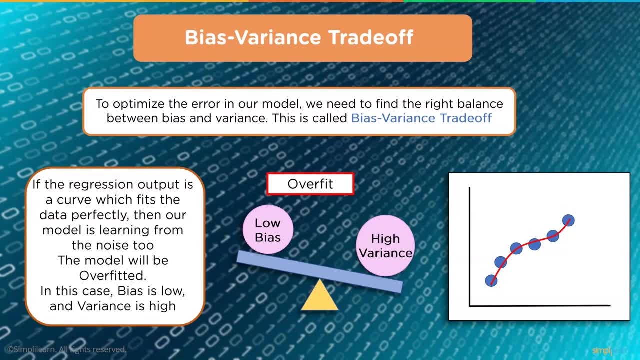 be the fact they both have fur And it might look at. all the Fox pictures had a little more fur And I'll explain that in a minute. cat pictures have a little less fur. That would be an overfitting kind of a visual example of an. 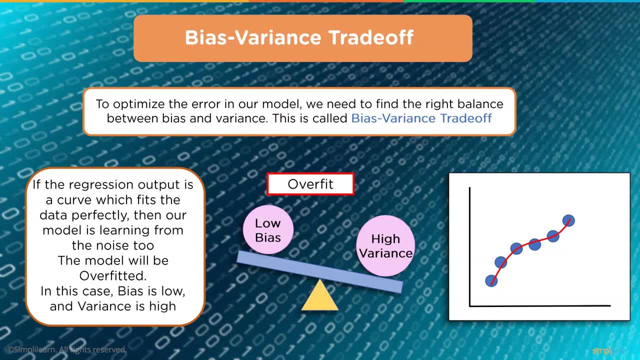 overfitting on there And you can see here we have the overfit, the lowest versus the bias, and it goes directly through all the points. There's no averaging out, there's no kind of generalization involved. The perfect fit for our data is a curve as shown. It fits to our data and disregards the. 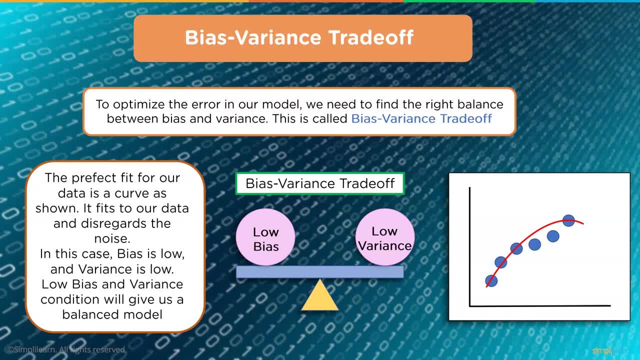 noise. In this case, bias is low and variance is low. Low bias and variance condition will give us a balanced model And you can see here a balanced variance trade-off: low bias versus low variance. Again, really, one of the things we're looking at is that we train the model as good as we can. 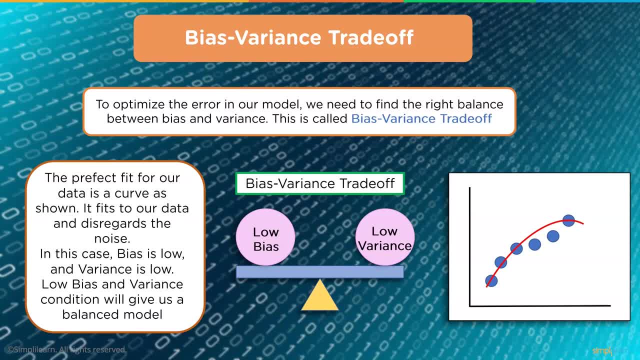 so that its prediction on unknown data and the prediction on its trained data kind of match with the same amount of error. That's kind of like we've hit the max, Anything else after that, we're just programming noise in there. Total error. The total error is defined. 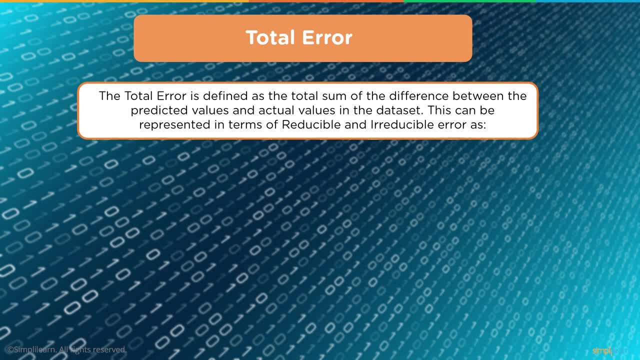 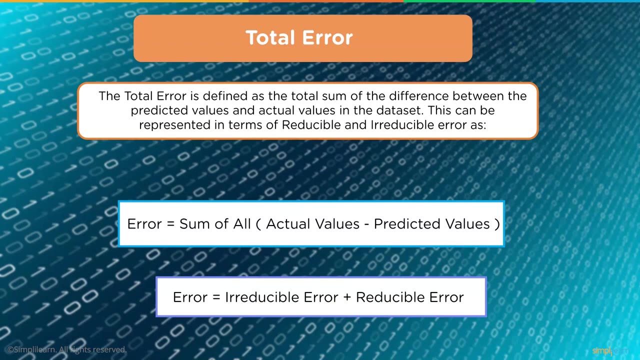 as the total sum of the difference between the predicted values and actual values in the data set. This can be represented in terms of reducible and irreducible error, as error equals the sum of all actual values minus predicted values. Error equals the irreducible error plus reducible error. 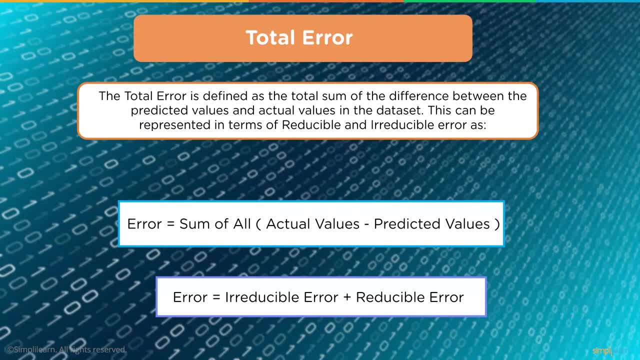 So keep in mind, when we start looking at error, it's usually where you start and you're working with your shareholders. Really, that bottom error that you show them is both of them, And so when you're presenting this to shareholders, really drawing the bottom line and saying, hey, we can't predict below this part and this is the 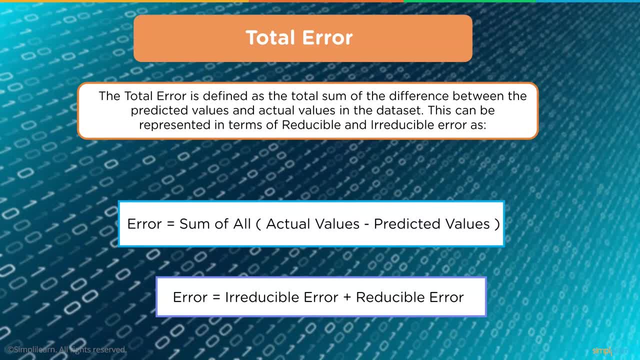 reducible part as we're coming down. This is what we're looking to find And it's really important because, as your models change and as you find better and better models to fit your data, really being able to see where these two separate helps a lot in finding a better model and a better 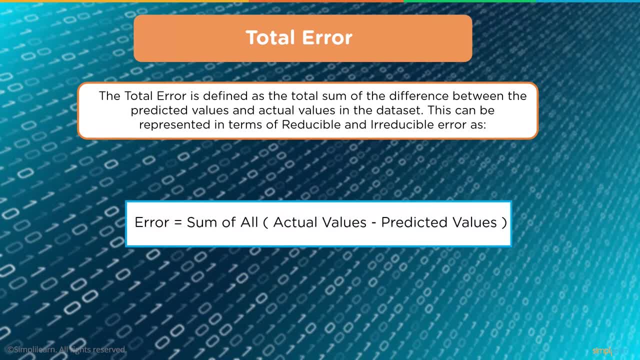 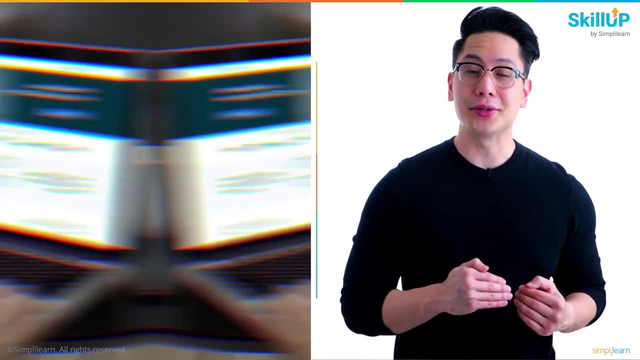 prediction Error equals sum of all actual values. predicted values Error equals the variance plus the bias squared. Getting your learning started is half the battle. What if you could do that for free? Visit SkillUp by SimplyLearn. Click on the link in the description to know more. 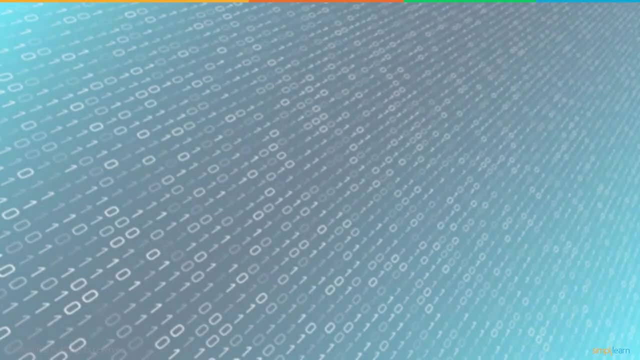 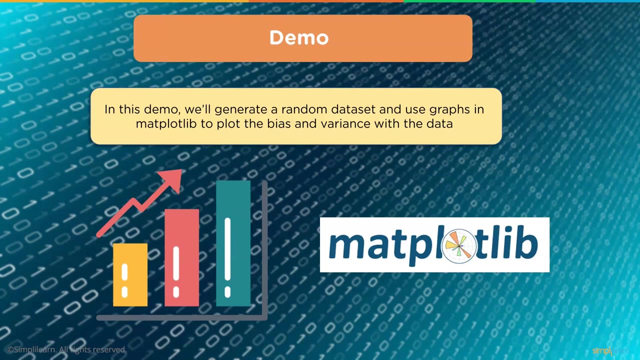 So let's go ahead and take a look at a hands-on for this, And in this demo we'll generate a random data set and use graphs and matplot library to plot the bias and variance with the data, And we'll be using Python. I always go through Anaconda and Jupyter for doing demos because it 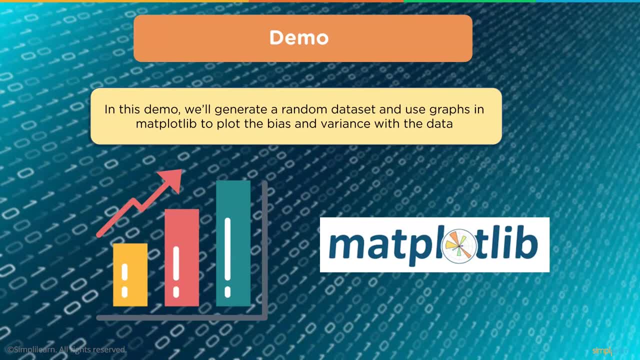 does a nice inline display. You can probably follow this with just about any Python IDE We're using. I think I'll either be in 3.6 or 3.8, depending on which setup I go under for the Python version. 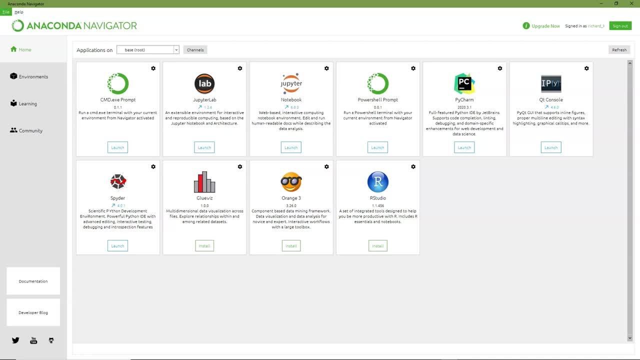 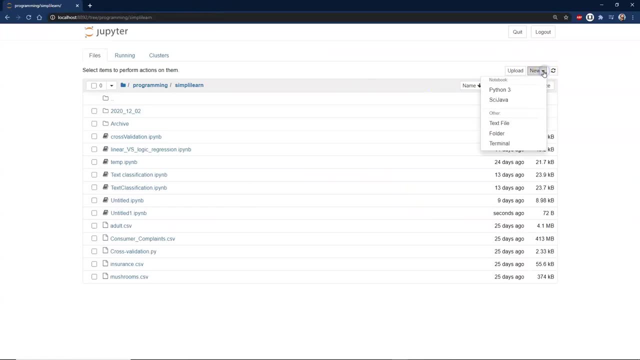 So here we open up our Jupyter or Anaconda, and then I'll go under the Jupyter notebook and go ahead and launch that. Once I've opened up my Python interface, which in this case is in Google Chrome, we'll go ahead and create a new Python 3.. 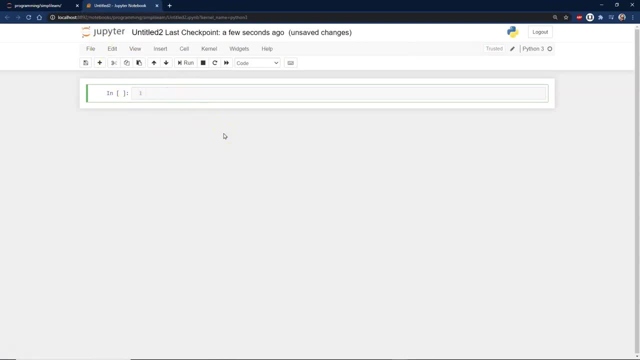 And once we're in the Python 3, let's go ahead and get our model going here In this demo. we're actually going to do two different little short demos here. This is just. this is like a lot of fun, So one of the cool things we can do. 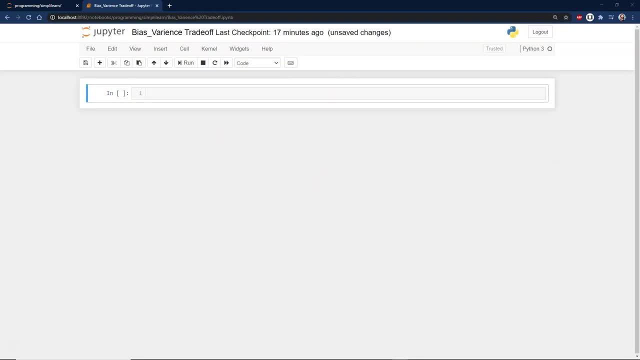 oops, it helps if I jumped ahead there as far as what we're working on. So this is one of those really fun things we can do. As you know, there's the NumPy module for your number array and we're going to take that NumPy module's NP and we're going to use our matplotlibrary. 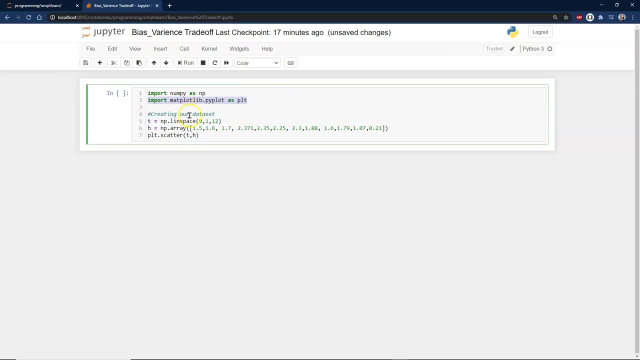 nice inline in the Jupyter notebook. If you're running this in a PyCharm, you'll find that it has a popup window And we're going to go ahead and create our data set And so we'll have our line space 1 to 12, and then you can see we put it in a nice array. 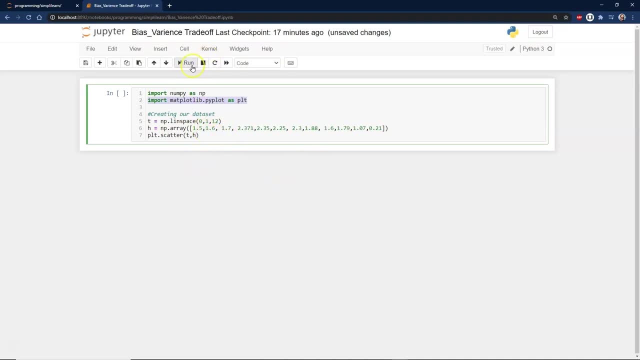 And we'll go ahead and plot this data so you can actually see what we're talking about. Let me just go ahead and run this. And so here we have our X value, if you will, which is your. this case, it's 0.2, 0.4, 0.6, so on. 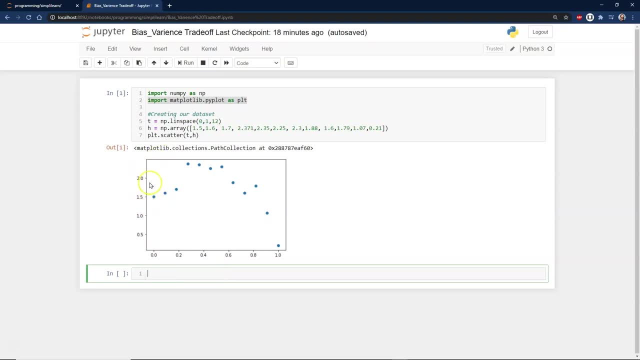 And then we have kind of a splattering of data going across. Now we went ahead and picked our data points, They did a bunch of random plots until they kind of had the data that looks like this, And we wanted to do that so that, as we do the rest of this little short demo before we get into one that actually uses some weather data, 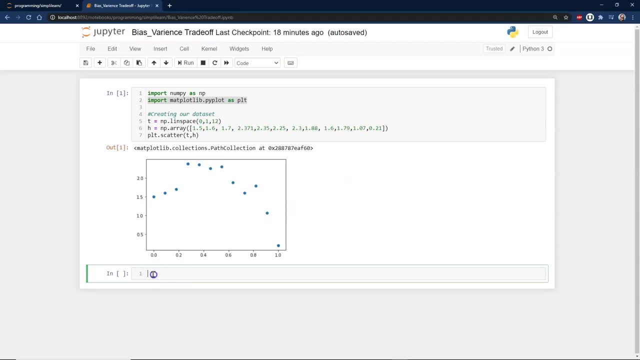 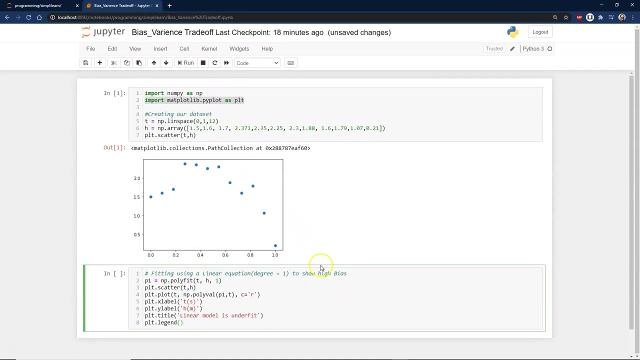 you have a little visual of what's going on here And we have a little bit more control over it, of course, So you can do this with random data if you wanted, and you'll see some interesting results. The first thing we're going to do is we're going to take and we're going to use the polyfit. 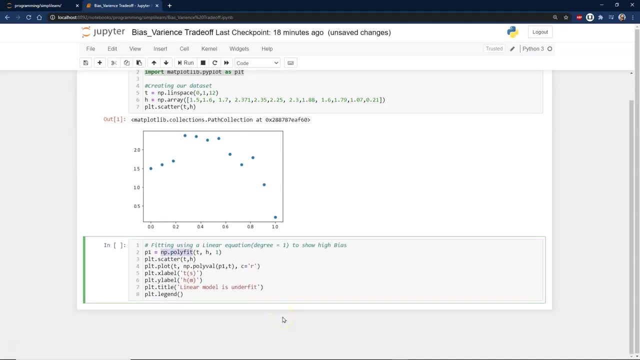 It's just going to fit this data to a polynomial function and it's going to be a degree 1.. So this is basically a Euclidean line. That's all we're doing is drawing a line based on this data, And so we're going to go ahead and plot that data and take a look at it. 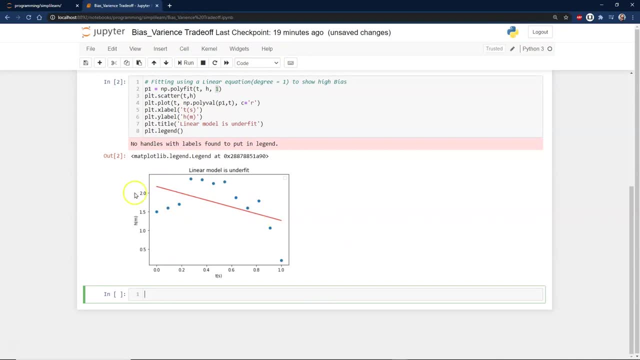 And you can see if we draw a line through the data, it really doesn't capture the data very well. As you put in the X number, your predicted value on the Y axis is going to really not connect very well. A lot of variance here. 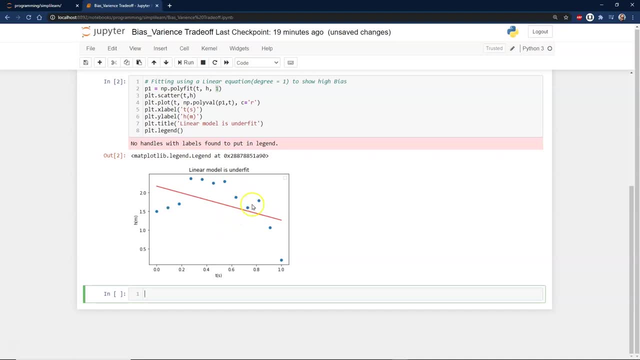 So we're looking at the setup on this where the variance is just high. This is kind of a bad model. So we're going to go ahead and plot that data to really view this data with and we can take a look at it and look at it the other direction. 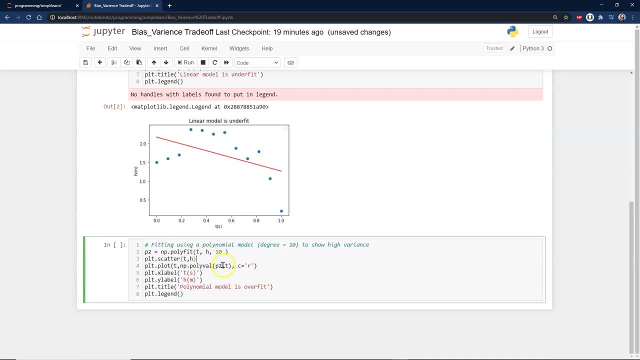 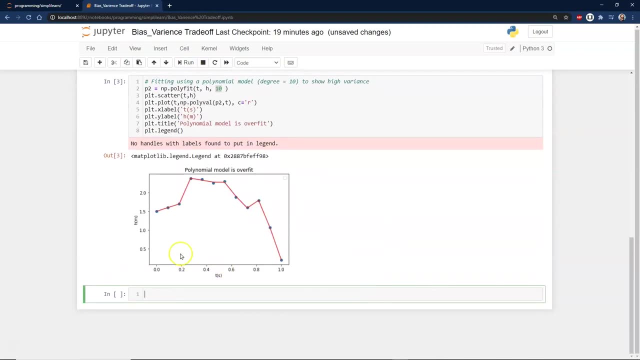 If you remember, we had overfitting. So in this case we're going to use a variance, We're going to actually use a degree 10 polynomial to fit this, And if we plot our level 10 polynomial on here, look how closely it fits the data. 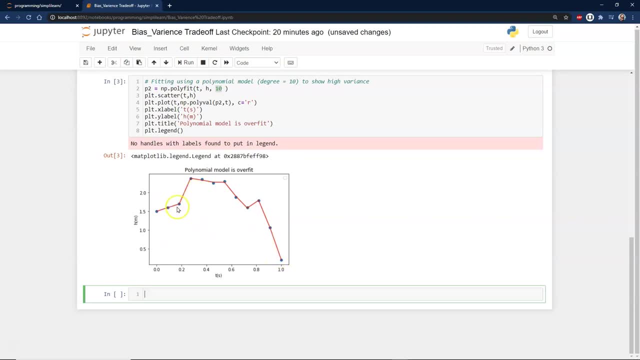 Now, if I was looking at this data just visually, you're going to guess that some of this is variances, right here, As far as the setup coming in, we just put a little drawing line there, Grab an arrow, There we go. 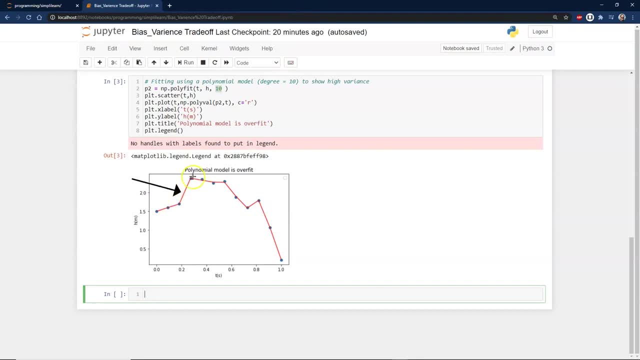 So we look right here, Look how this just jumps, And then from here to here you have a line and a jump and another line. It really jumps around. I would just looking at it- it's almost painful to look at it and think of this as predictive values. 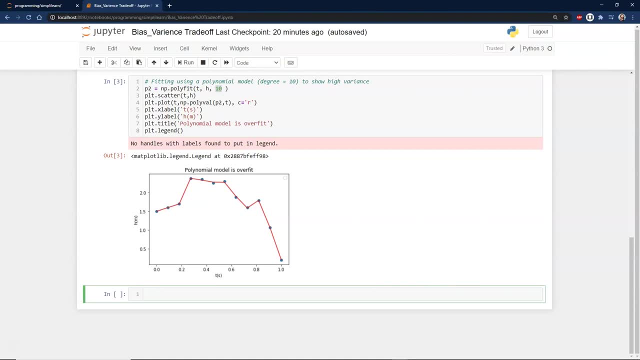 As far as getting enough generalization to capture New data coming in, And so we're going to go one more. Like I said, this is just a brief look at what we're talking about, And we're going to have it do a polynomial degree 2.. 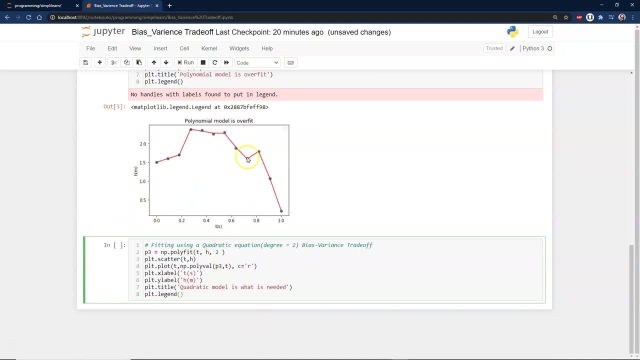 Well, what's a polynomial degree 2? It's hyperbole And it's either going to be aimed up or aimed down. You look at this. you'd be looking at a minus a times x squared plus b, or something like that. 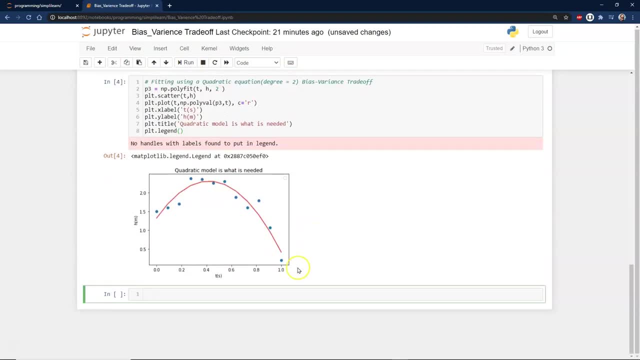 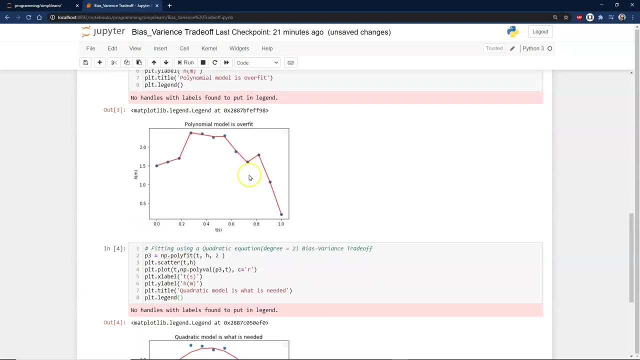 So let's go ahead and run that with a hyperbole And look how nicely it fits the data here. It's got a little variance, But if I was going to pick from these three different formulas, I'd definitely go with the third one here. 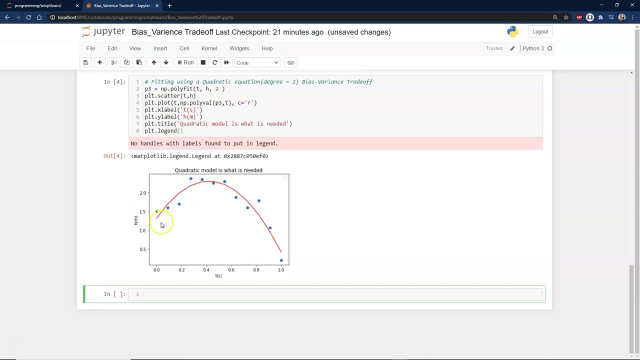 Because it goes right through a lot of the data And, as a generalization, it looks like a pretty good rule for predicting what's going to happen, depending on your x value, And if you put another value in here, you'd get a pretty good guess if it continued with the same format. 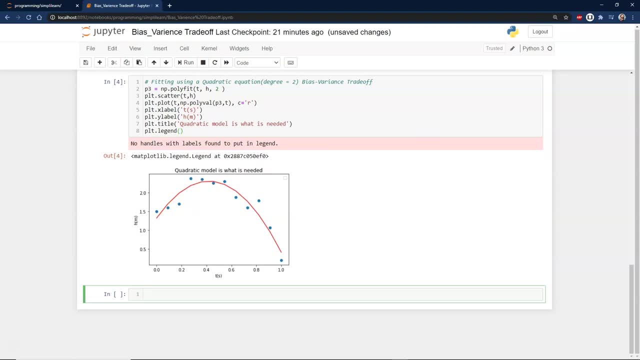 So this is looking at it where we controlled the data And you can see the polynomial fit from here And you can see the polynomial fit from an NP numpy array, the NP array. Let's take a look at this and actually put it to some data on here. 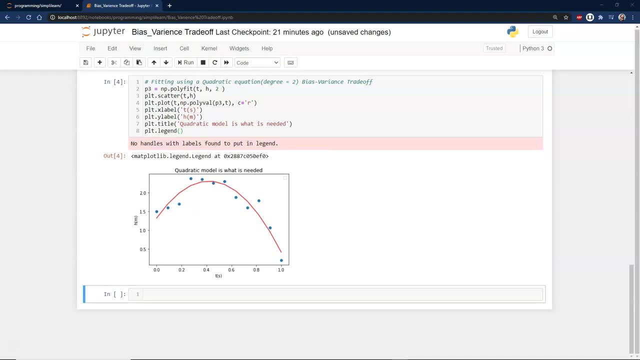 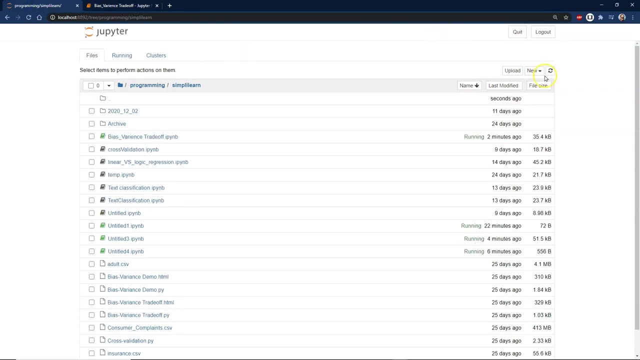 And we're going to use the weather station as far as like a format. It's always fun to bring in some new data on this And let's take a look at that. Let me go ahead and create a new. Let's see. 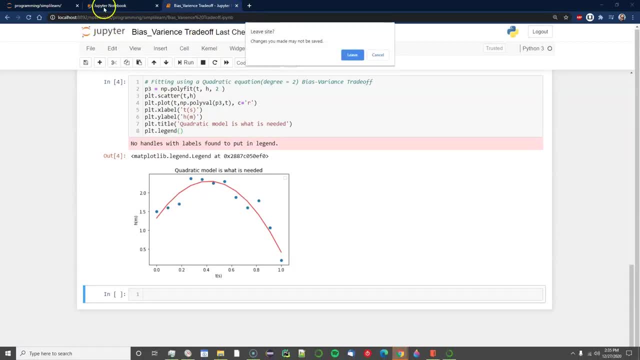 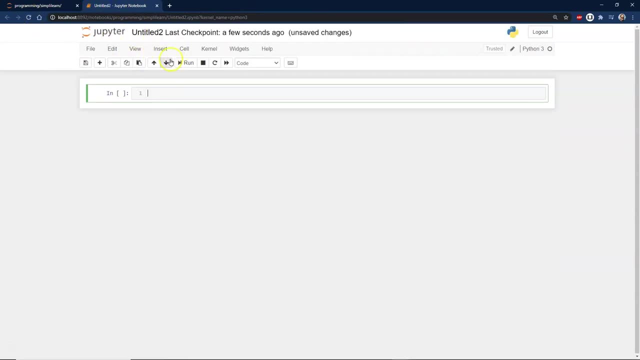 Here we go: New Python 3. Go ahead and close out this one. we just did: Oh yeah, Leave, And let's go ahead and go in here and take a look at something different. So for this one, we'll go ahead and use our pandas, just because it makes reading files really easy and quick. 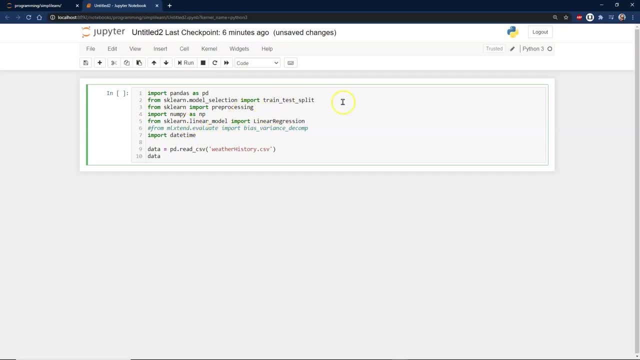 We're going to be looking at our SK model selection, import train and split. A lot of this- if you're at this level already talking about bias and variance- should all look familiar when working with sklearn. We're going to do some preprocessing stuff on the data. 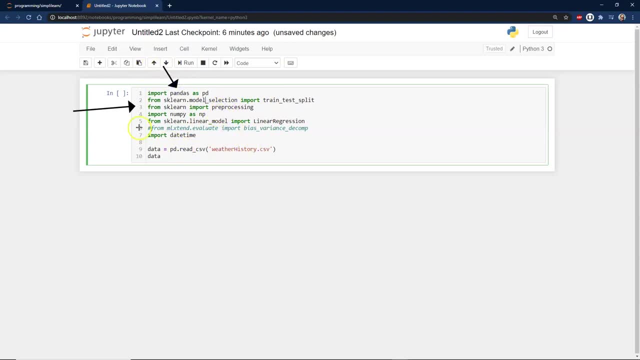 Let me put an arrow up here for our pandas. And then of course, here's our numpy setup. here You almost always see pandas and numpy together, since pandas sits on numpy And we use numpy for a lot of things. In this case we'll actually be using the sklearn linear regression model. 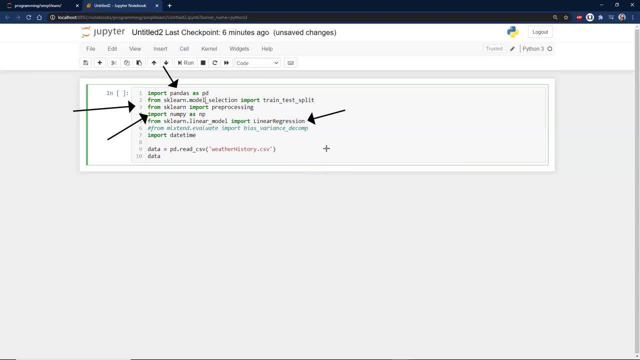 By the way, the linear regression model for most data going in, if it's just raw numbers and depending on what, if there's not like a split in features of true, false and things like that, the linear regression model is one of those. 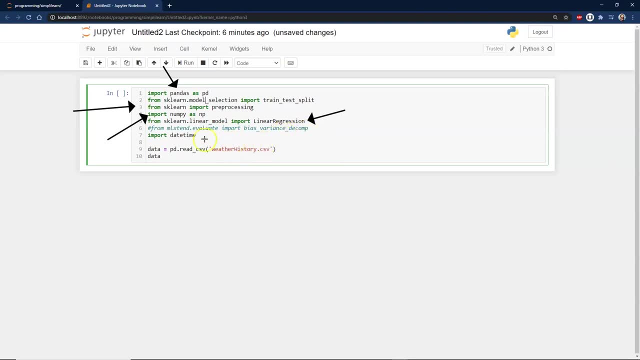 It's just so powerful. And then date time. I think some of the data has a date time stamp on it. Sometimes we just import it. because it's a habit When I'm doing really large data pools, I put a timer at the beginning, at the end, because I might be doing the first hundred out of three thousand. 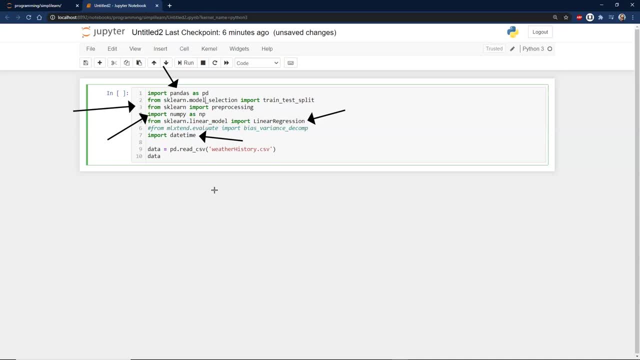 And if that takes an hour to go through all that data because each one of those is a huge file, then I can guess that. or if it takes like a minute, well that's three hundred minutes, So that's a couple hours, And if I'm going to run it on three thousand, I want to start looking at multiprocessors and things like that. 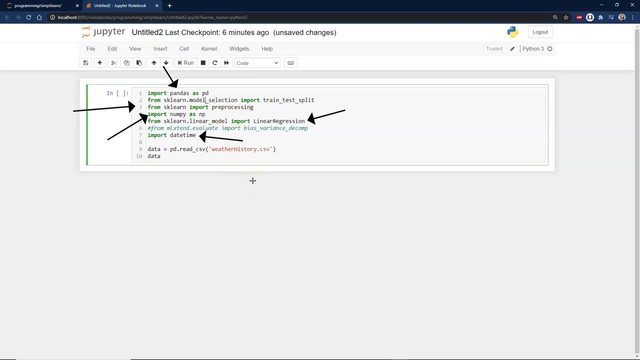 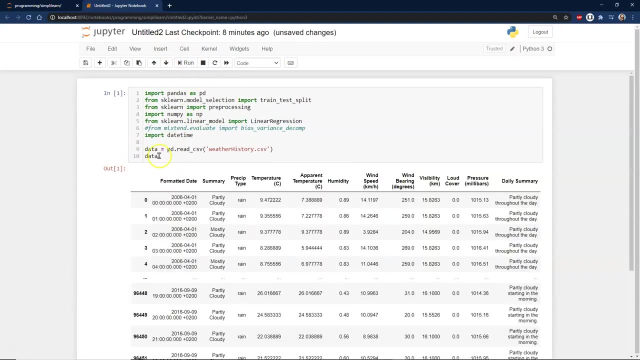 So again, these are things that we just kind of bring into our setup And we'll go ahead and run that. so they're all nice and neatly loaded. And then we did just straight data. If you put your variable down here in a Jupyter notebook, it does a nice job of printing it. 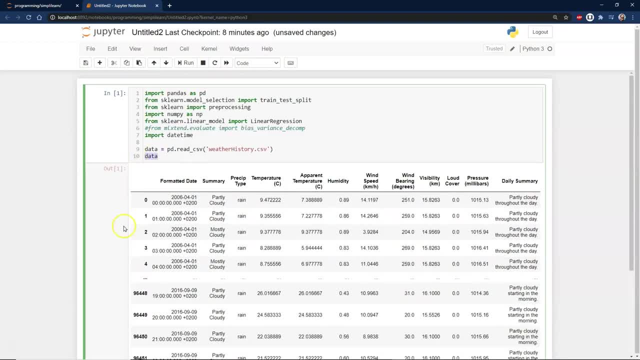 You can also wrap it in a print statement. It's always the last piece of data you put on there that it prints. If you put a bunch on that, it'll only print the last one. So this is the data we're looking at. 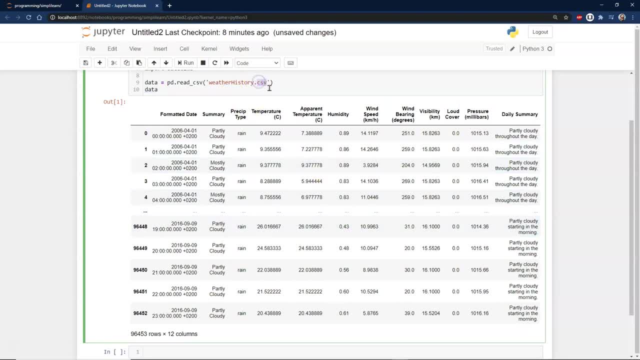 This is the weather history comma separated variable file. Of course, you can always put a note in our YouTube or send a note back to the team if you don't have a copy of this file and you want them to send you a copy and more information. 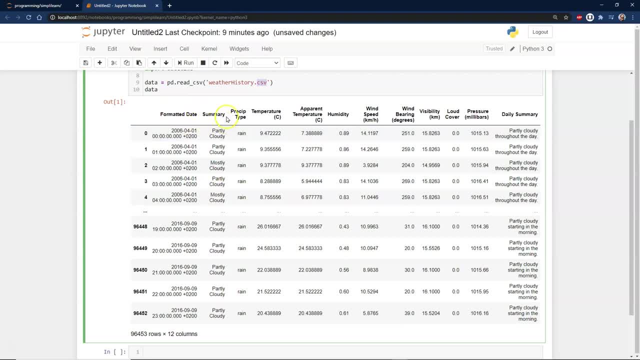 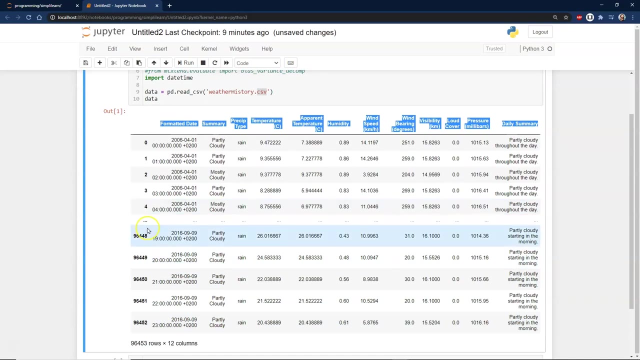 And you can see, here we have our formatted date, our summary precip: type, temperature, apparent temperature, humidity, all these different variables that they're picking up off of their different weather instruments. And I happen to live near NCAR National Center for Atmospheric Research. 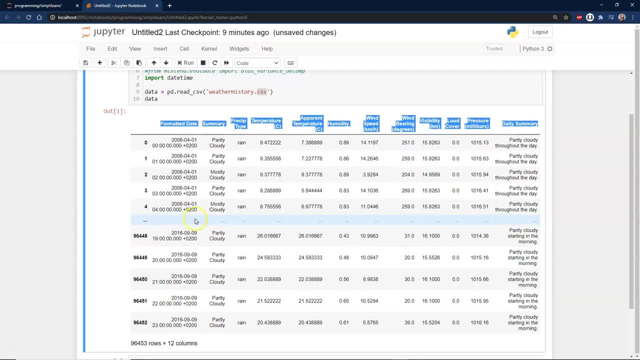 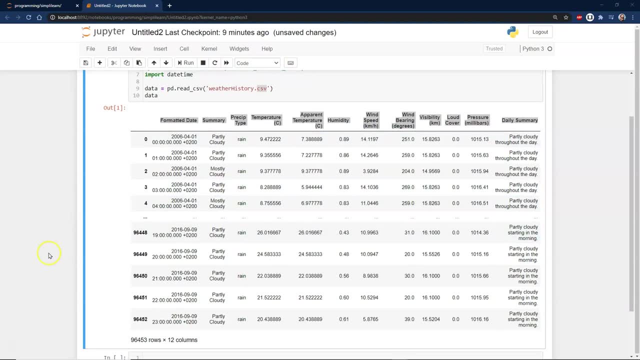 They collect so much data It's mind boggling. They don't even know what most of the data they collect means. In fact, there's so much data that is untouched and they're still digging through all the features to figure out how these different measurements work. 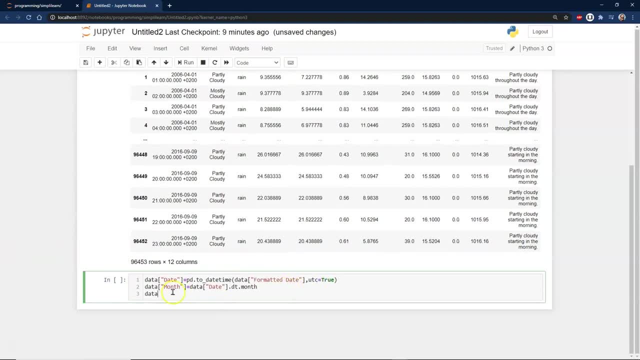 So as we start going into that, we're going to spend a little time. I don't want to spend too much time on this next part, explaining it, Just to give you a feel of some of the stuff that goes on. I was originally going to take this out and just put it all in one set of line statements. 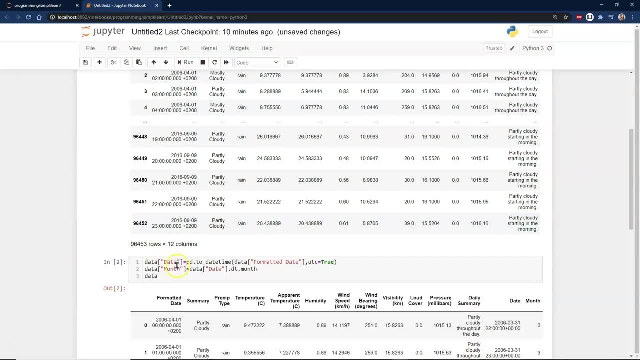 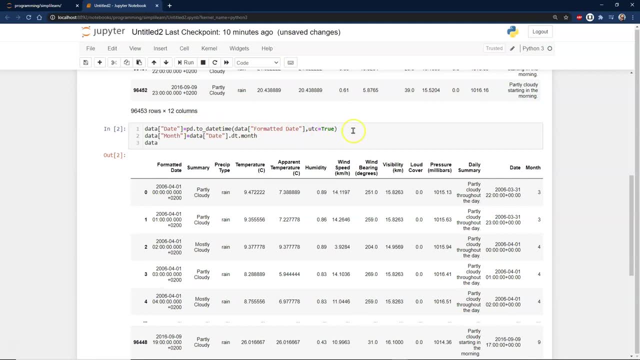 But as a data scientist, 80% of your work is cleaning up the data, And so here we have our date. We're going to switch that to formatted because you know you kind of want your date to switch around a little bit. 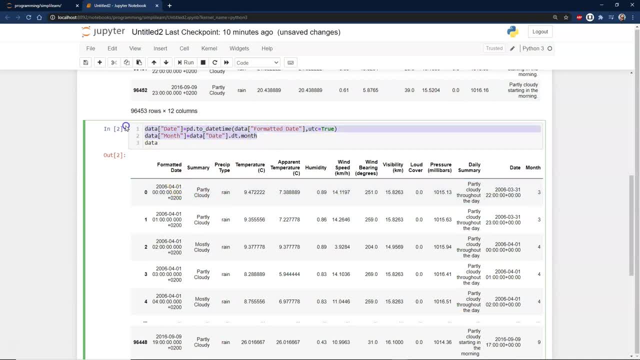 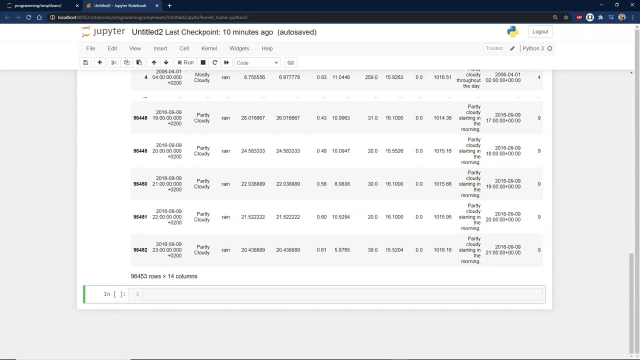 Formatted date, month, date, date, date, month. So we're just meshing with the date information there and then double checking it on our printout, And the next step we might want to go through is take a look at some of the stuff we might want to drop. 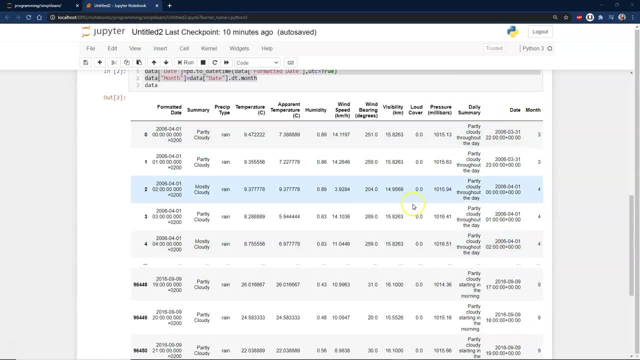 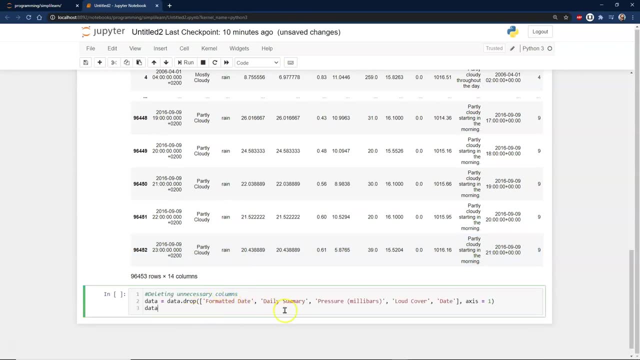 Because we just here we go, You can see here, here's the date and month at the end, So we really don't need the formatted date anymore. It's just a character string. So we're going to go ahead and drop that. 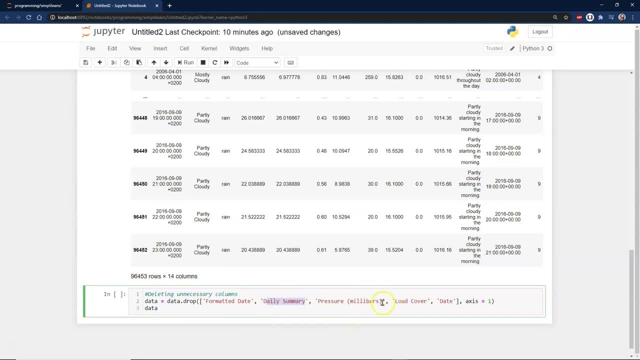 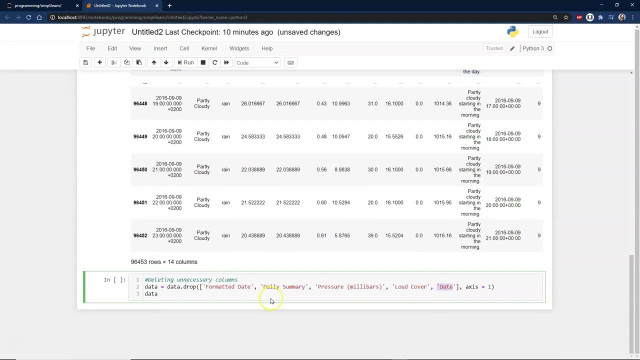 We're going to drop the daily summary, the pressure and millibars loud cover, And let's drop the date too. So we're just going to have the month on the end And we'll print that out again and run it. 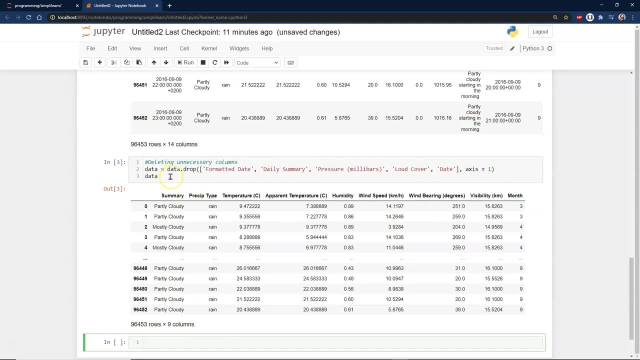 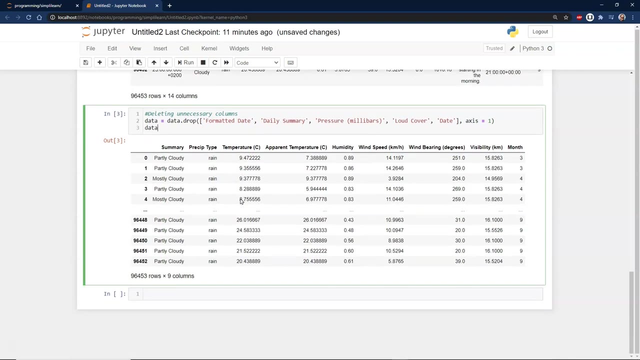 Again, these things are more of a domain specific, Very specific to weather and what you're looking at. You could probably do a cross validation or feature selection kind of setup in here to figure out what you're looking at. We're not going to spend time on that because we're really focused on, in this case, the bias and the variance on here. 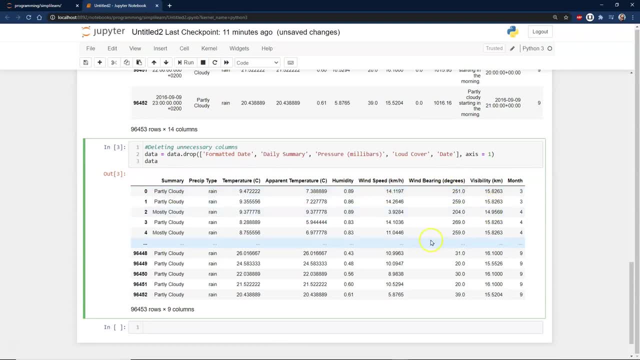 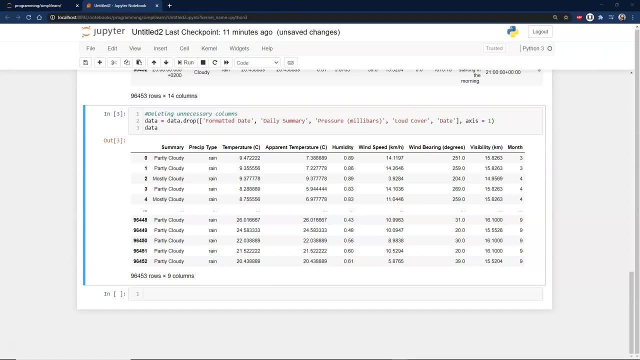 So, okay, we've cleaned up a little bit of our data. as we look down at it, One of the things we probably want to go ahead and do is do an encoder, So anything that has like a label. In this case, we have what rain. 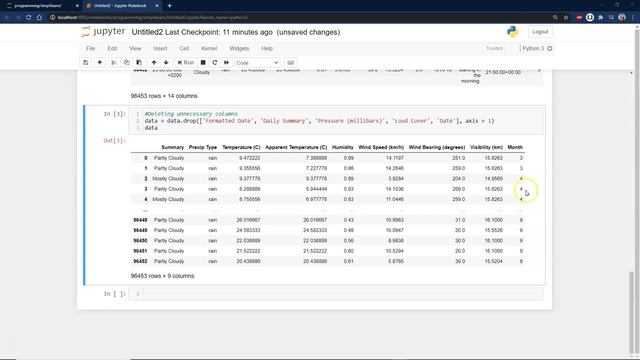 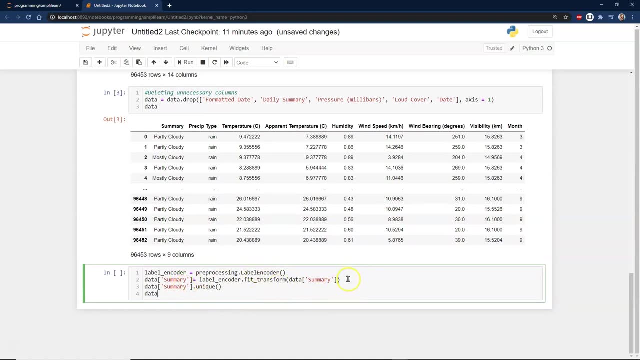 Precipitation type. that'd be something that'll be running through an encoder. Let's go ahead and do that on here: Pre-processing encoder, And so the summary label fit: transform summary. Let's see where is our yeah, summary. 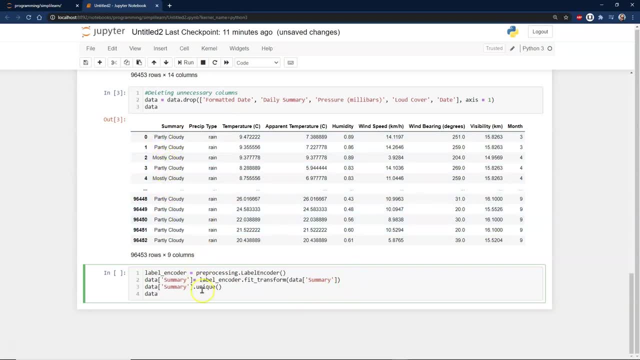 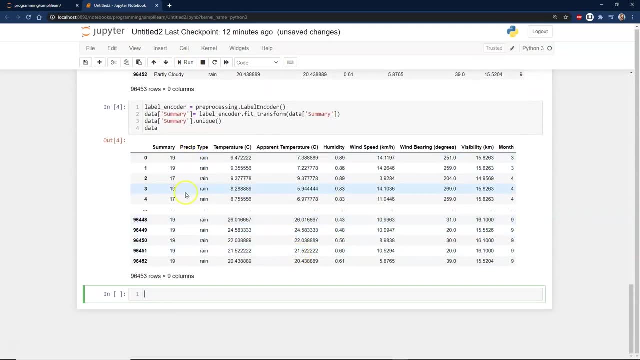 Partially cloudy, Mostly cloudy. We want to go ahead and do an encoder for that, Make sure it's unique on there And run that And then print the data out again And you can see now. summary is 19,, 17,, 17.. 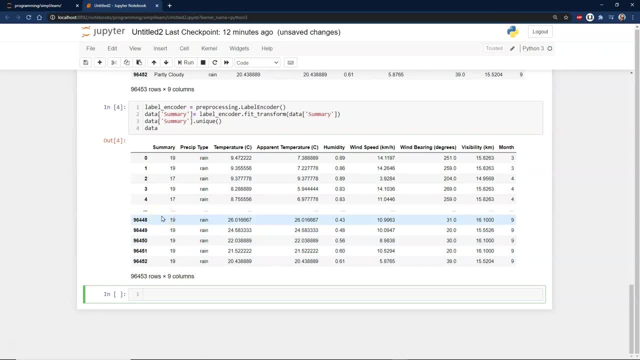 So it's giving it a nice integer value for as far as the summary setup on there. And then there's also precipitation type. That's the one I noticed. first. They went for the summary first, our guys in the back, So we have rain and snow. 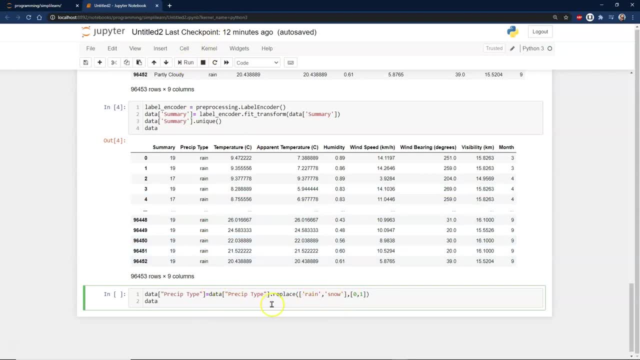 We want to look at that and go ahead and take that and switch it around. Precipitation type: replace rain and snow with 01.. Go ahead and run that And there we go. Precipitation type 0.. We have our summary. 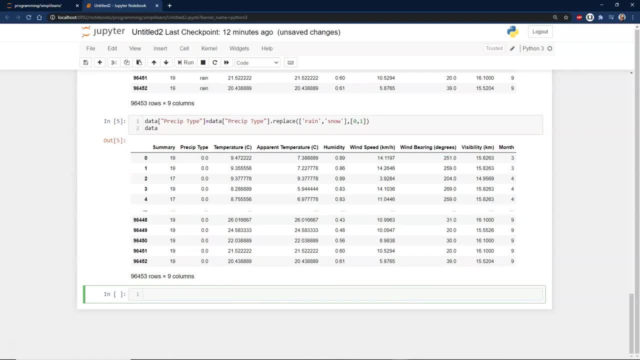 That's all nice in integers. Looking across, Double check everything And if you'll notice on here one of the things you'll see- data. We want to go ahead and check for null values, So let's go ahead and put that in here. 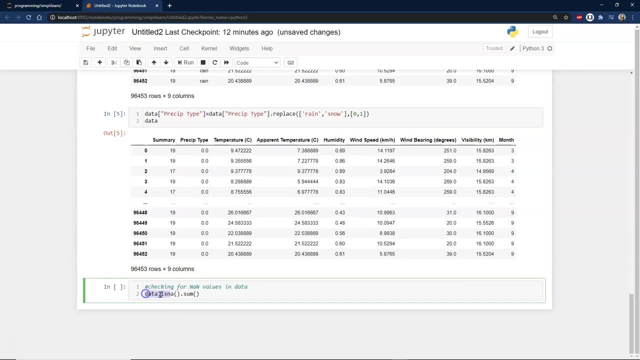 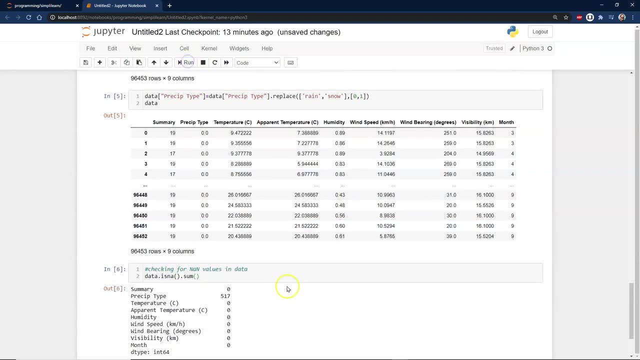 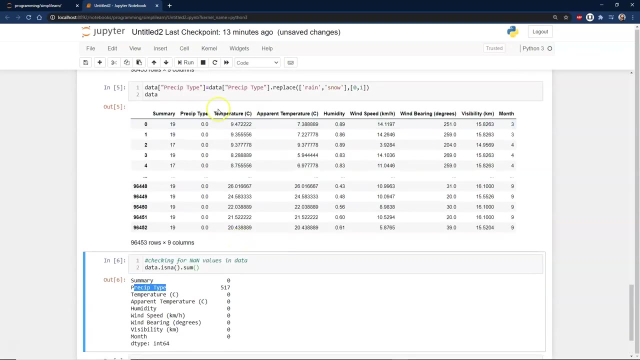 Data is in A. This is our, remember. our data is a pandas. This is a pandas checking for null values And we're going to summarize it, And it does it by each column. Look at: this Precipitation type has 517 null values. 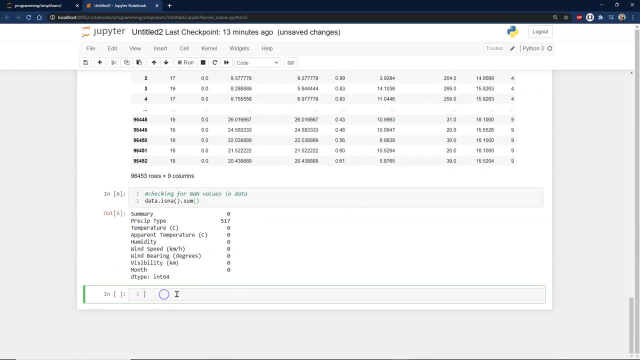 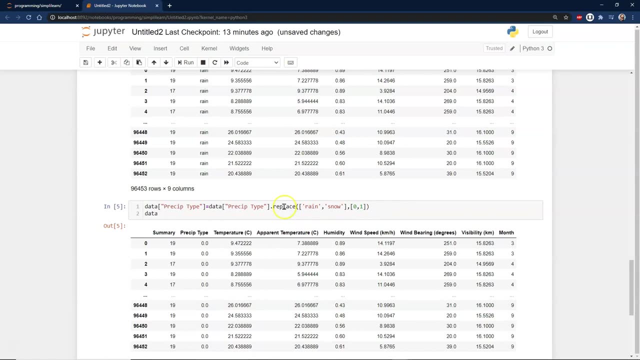 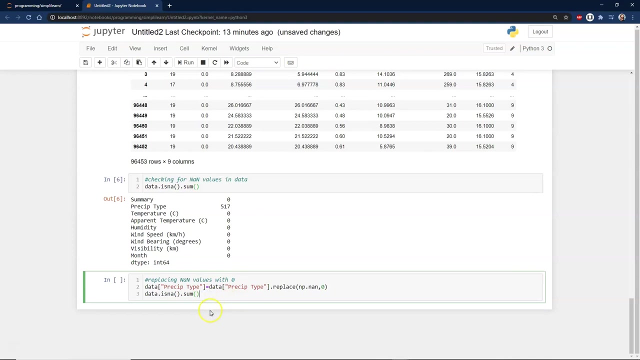 That's going to cause an issue, So we want to go ahead and fix that. And again, I'm not spending a lot of time on this Because this is pre-processing Data, is really digging in here to this specific data, And so we want to focus a little bit more on the end result. 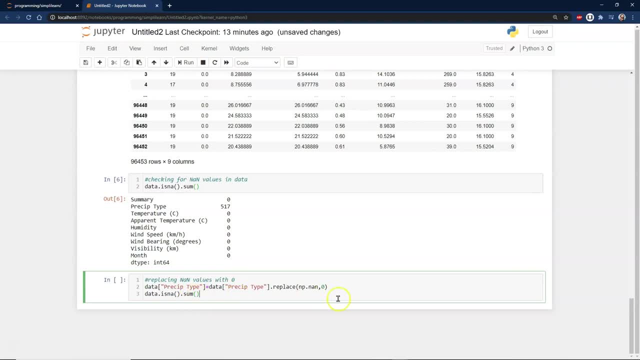 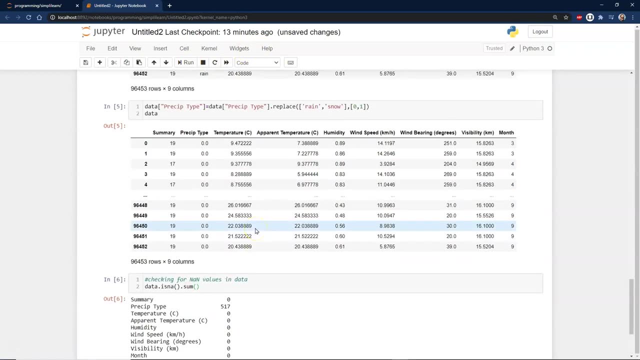 And then we're going to go ahead and take our precipitation and replace it with a 0. So any place there's a null value, we want to put a 0 in there. We'll go ahead and run that, And now we have our sum. 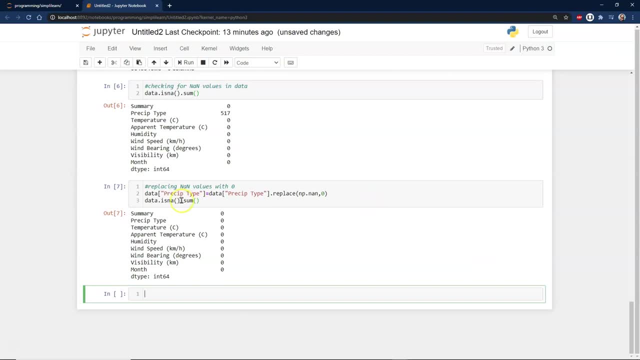 There's no null values. We went ahead and took care of that. I have a feeling that if I dug deep, this last step was probably incorrect, Only because I have a feeling that when we did the 0, 1 underneath precipitation type. 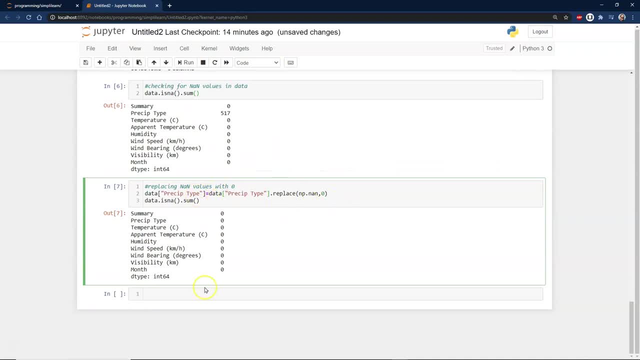 that there might have been a third value And that that's what gave us the null values. I could be wrong Again. I'd have to dig through hundreds of lines of data For this demo- probably not, But if you're on your own time, you might spend a little time trying to figure out what we did right here. 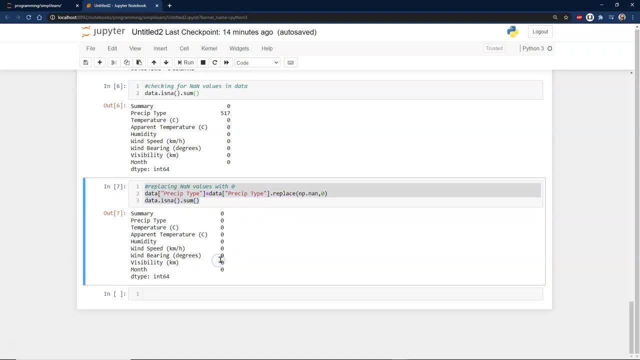 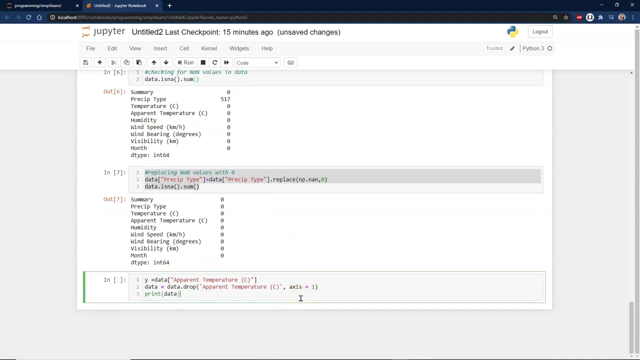 And why it's probably wrong. But for this this is going to work just fine for what we're looking at. And now we dive into the fun part. Formatting data to me is also fun: Digging through the data and finding out where the null values is and what it means. 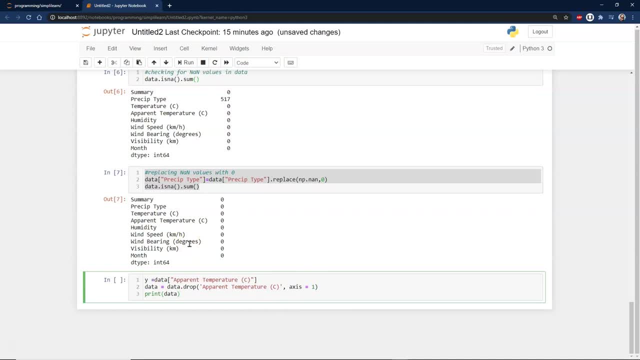 That's a different kind of fun. It's very domain specific. So I usually find myself learning something new When I look through really intensely. look at the data. This is the part where we're starting to talk about the data science. So here we have Y. 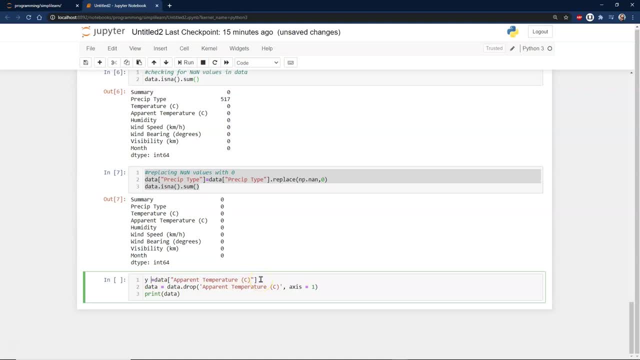 We're going to look at apparent temperature C. That's what is going to be our. this is the column we want to use for our Y. There's our Y value, And then we're going to go ahead and take that same column and drop it from our data. 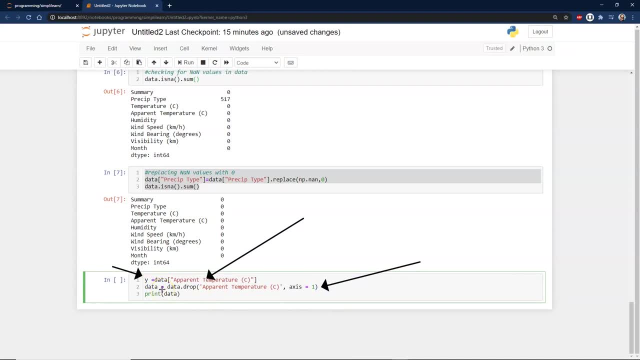 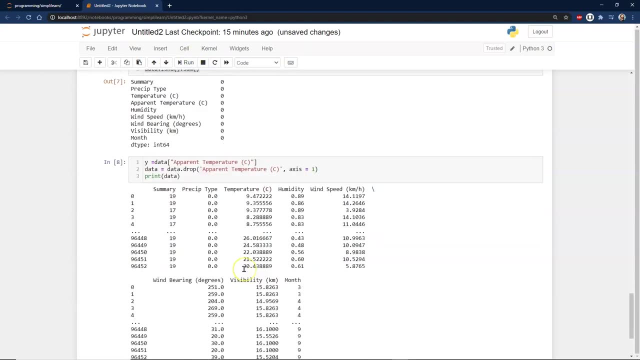 So we have our Y value and our data. Let's go ahead and do that. You could say our data is going to be our X data. So we have our Y data and our X data. So we go ahead and drop that And you can see right here when we print the data, we no longer have the apparent temperature C. 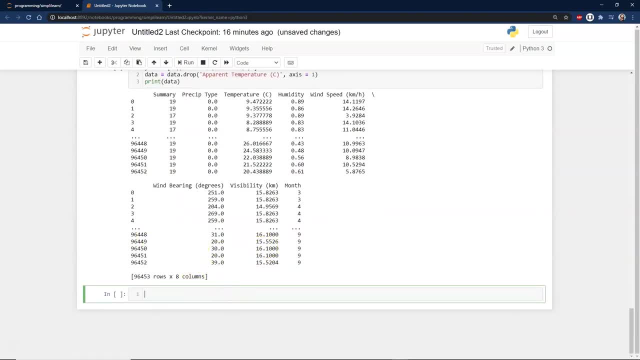 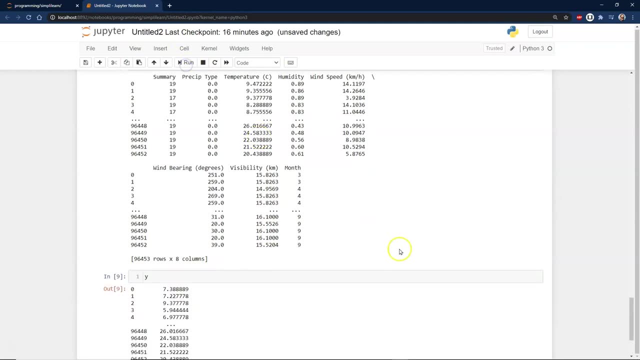 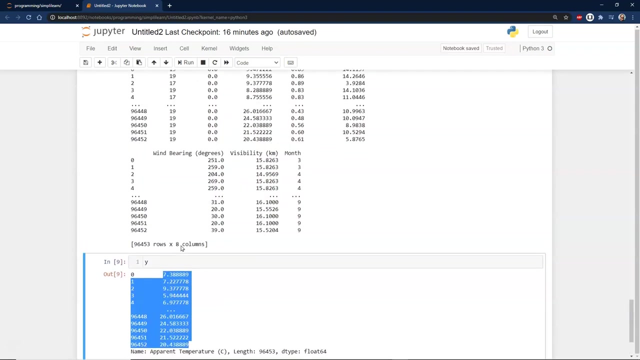 It's gone out of here. That's now going to be our Y value that we're trying to predict, And if we just type in Y and run that, These are the values that we want to try to figure out. We want to guess what the apparent temperature is going to be based on the other information. 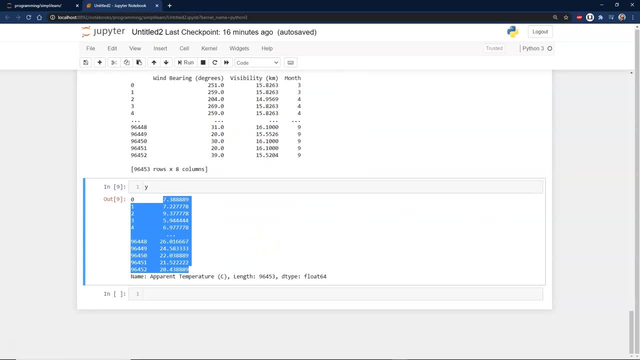 That's what we're looking for, And, of course, you could switch this around. You could be looking to see if the temperature is going to be predicting the rain. There's all kinds of things you could do on here, depending on how much fun you want to have and how deep you want to dig into this model. 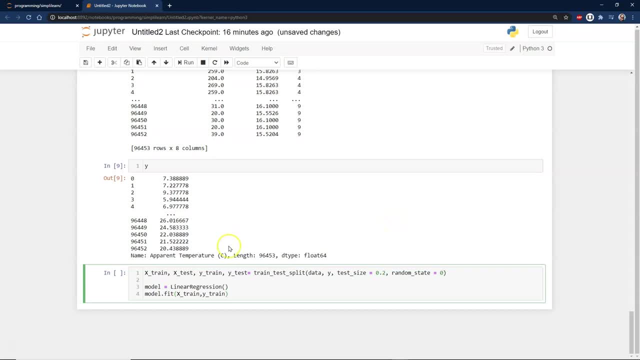 And here we're splitting our data. This should all look familiar now. We have X train, X text, Y train, Y test Train test split. We have our data and our Y going in. Let me just put an arrow right there. 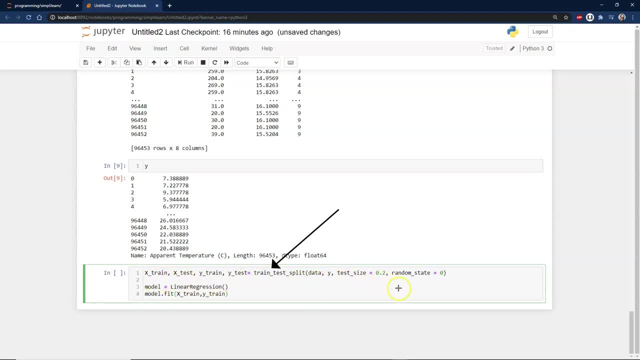 On this part is the one we're looking at, And so we're going to do test size 0.2.. So 20% we're going to use for test, Random state equals 0.. Not really too worried about that in this example. 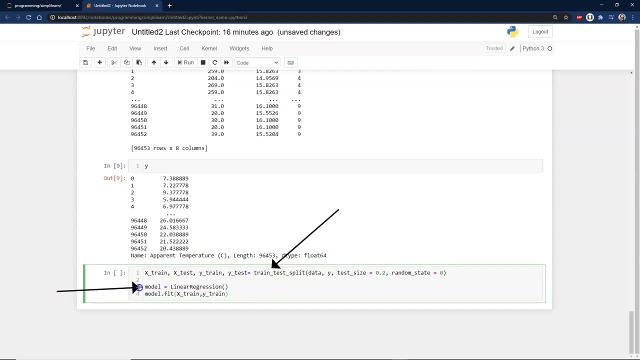 And then we said we were going to use the linear regression model from sklearn, Because that's a really powerful model for dealing with numbers And we're dealing mostly with numbers And then we're just right off the bat going to fit our data to it. 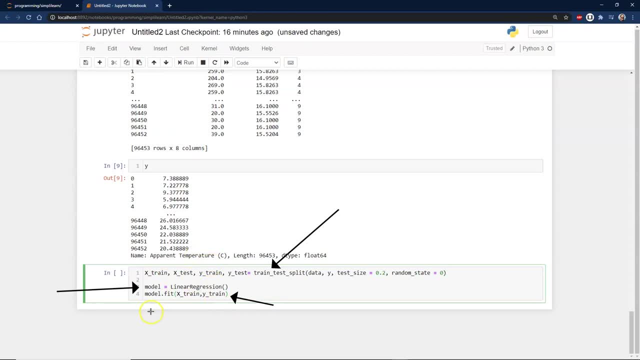 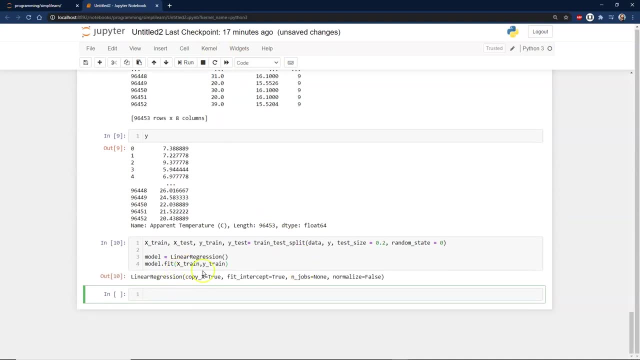 So we're going to take our X train and our Y train and we're going to fit the model And let's go ahead and run that And you can see we've created a linear regression. Fit, intercept equals true and so forth. That's just letting us know our model is there and valid. 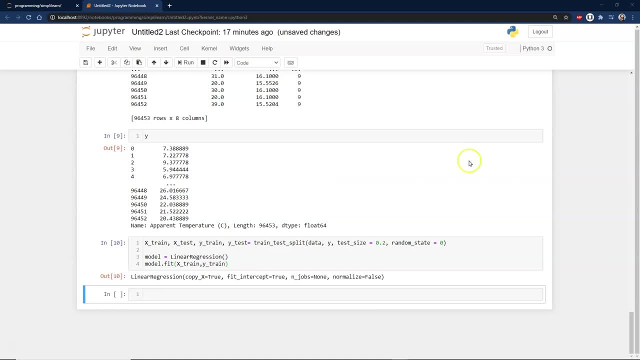 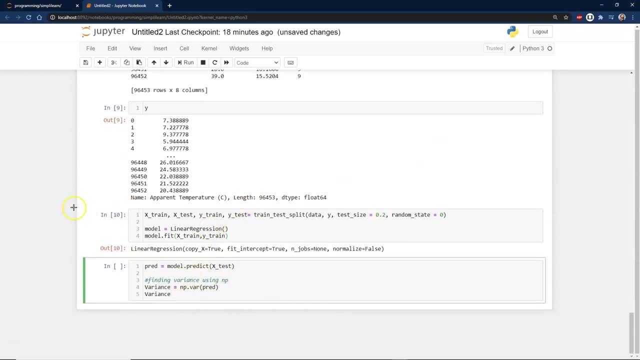 Now, from here, we want to go ahead and run our prediction on our test data. So remember, it hasn't seen the test data Here. we did our training and we fit our data. I call it training, but it's fitting the data is how sklearn refers to it. 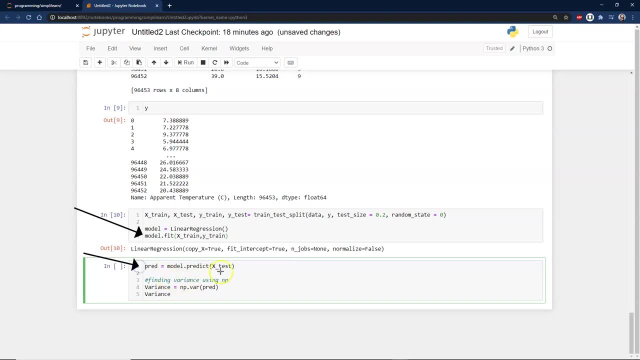 And then here we want to go ahead and get our prediction, So we know what the answer is, because we've already split the data. But this model has never seen this X test data before, And we want to go ahead and look at the numpy variance. 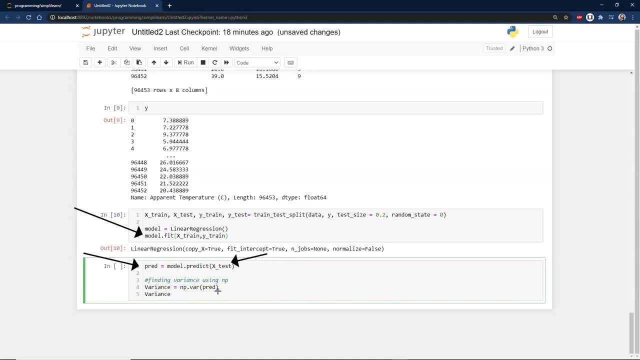 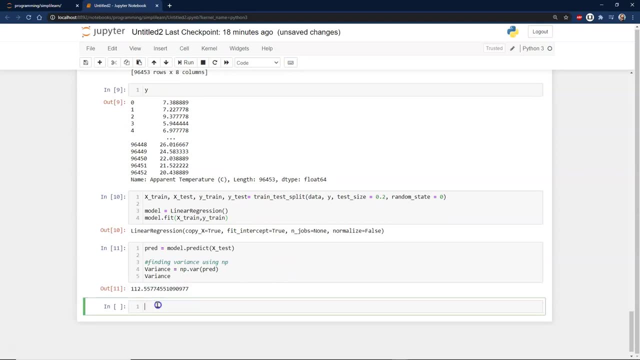 And we'll just push the prediction right into numpy variance And we're going to see how much variance there is in this data And let's go ahead and run that And you can see right here it generates kind of a number. These numbers are hard to read because this variance is based on the data coming out. 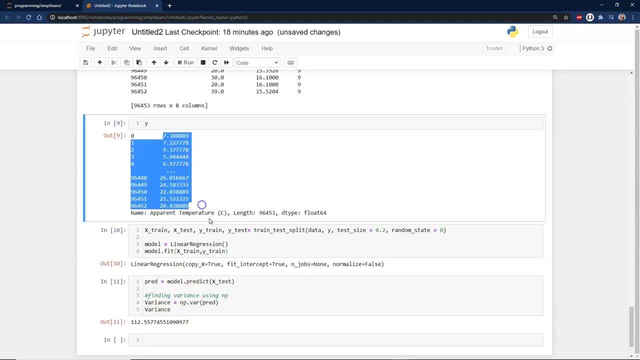 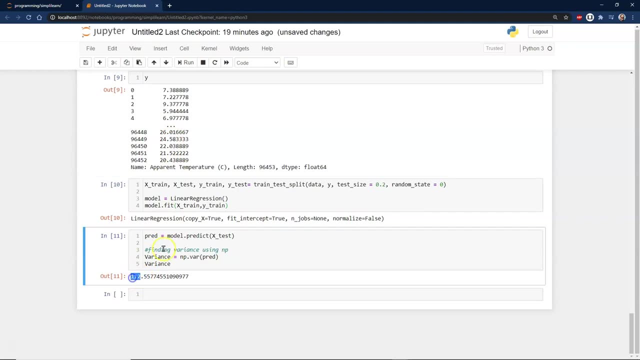 This is actually a pretty high variance. You'll see, right here is our Y and it's coming out and saying 112.. You look at a lot of these values are 26,, 24.. So this is a very high variance on here. 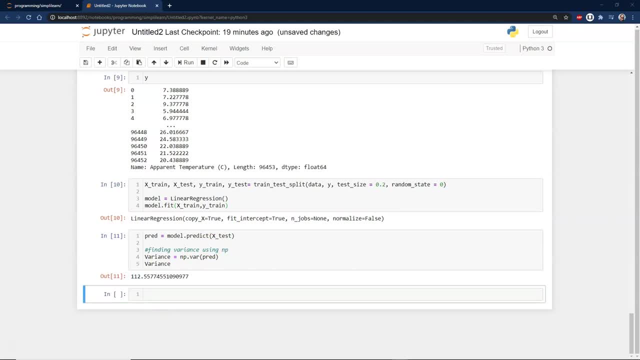 These values coming out are pretty high And we can go ahead and look at the bias on here And, if you remember from that last formula, we want to go ahead and find the squared value. This is the let's go back to that slide, so it helps. 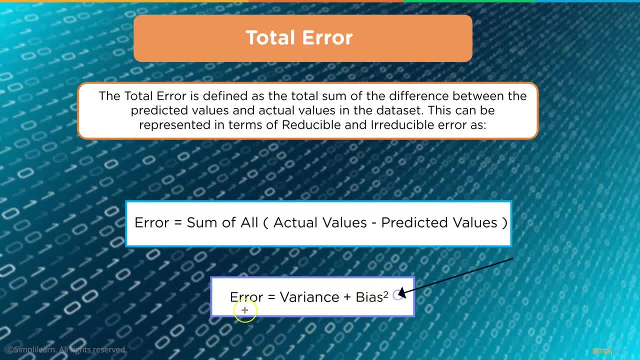 And so you can see on this slide right here we have the error: equals the variance plus the bias squared, And that's where this formula is coming in from. numpy Is looking at that bias squared. We can go ahead and switch back there. There we go. 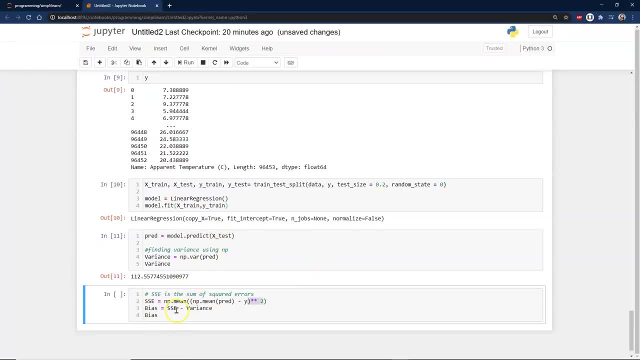 So when we're in here, you can see, right here is our bias equals our SSE, which is our error, And we want to go ahead and take the bias. We want to go ahead and take the variance. Well, you can see, here, SSE equals the mean. 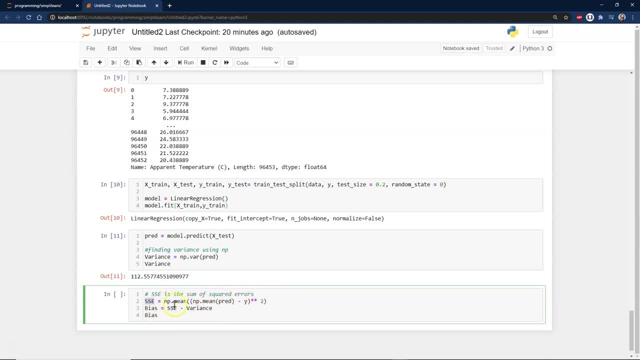 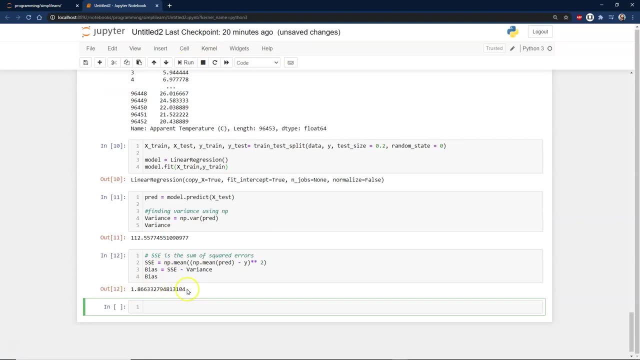 Mean minus Y times 2.. And the bias is the SSE minus the variance. And we'll go ahead and run here and print the bias out And you'll see we have a bias of 1.86.. And so when we start looking at these numbers, we start looking at this. here is a very large number. 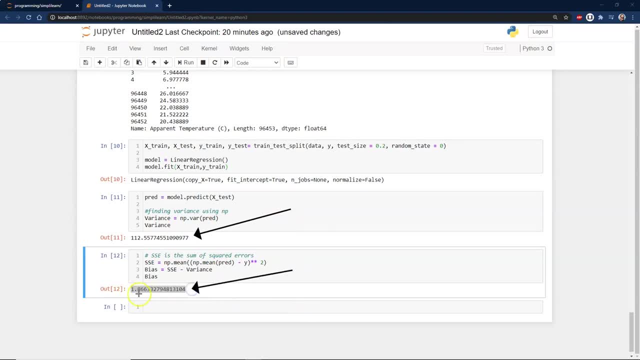 And we come down here and we see that our bias is pretty small And we can see- we're also looking at these numbers- here is our Y value coming in, And so in comparison, when you put these three together, our variance is still pretty high. 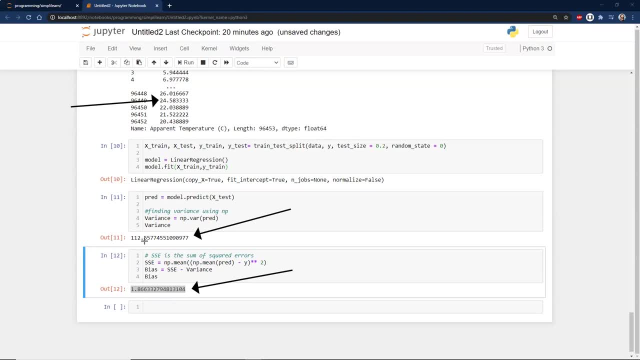 There's a lot of randomness in weather. Remember I was talking about you don't know which way the wind's blowing. You know you can stand there and say it's a windy day, But to actually guess how you know when the gust of wind is going to hit next and how it oscillates from moment to moment, is almost impossible. 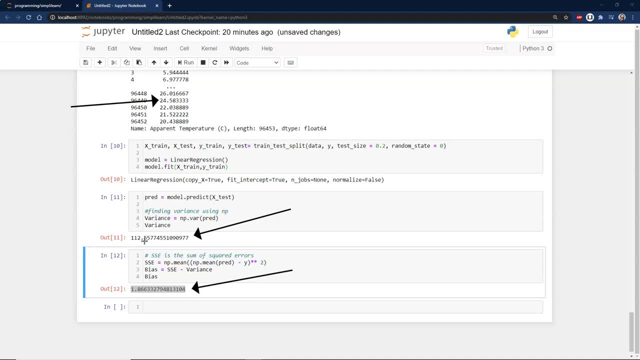 It's really hard to do. If you ever want to try it, go out there and stand in a windy day And you can see here that we're looking at temperatures and things like that and weather. It's the same thing. There is a lot of variance in this. 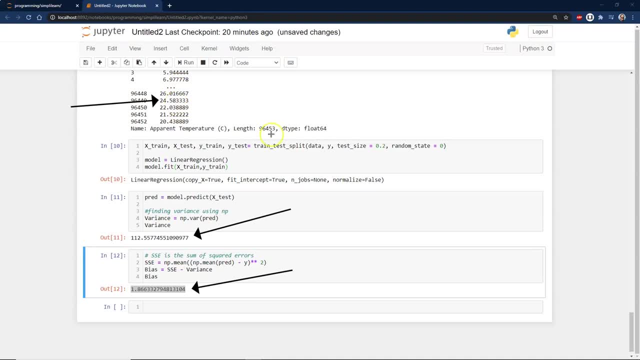 So this is why a meteorologist can be within 50 percent And 50 percent of predicting the correct temperature coming up, and they still get to keep their job. That's the job I want. You know 50 percent accuracy and you still get to work there.